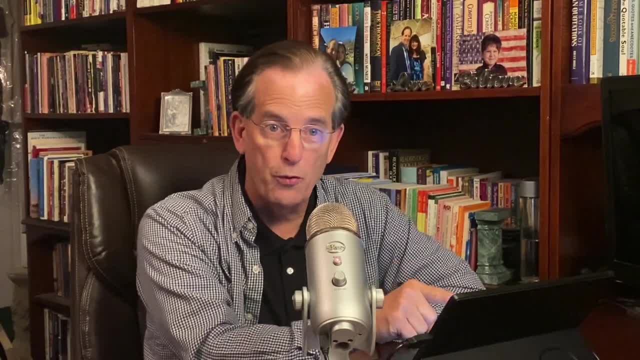 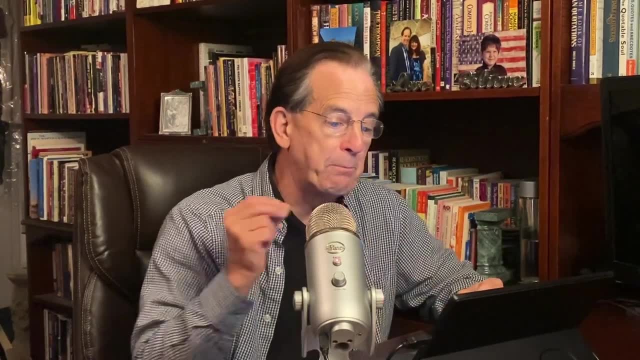 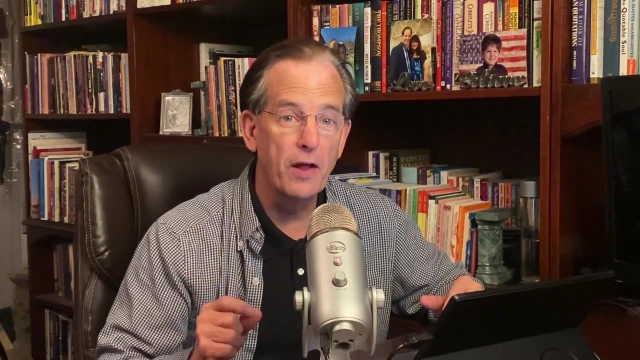 I happened to read on the internet this quote from EckhartYogacom. It says: As a way of connecting to, revering and paying respect to deities, many yoga postures represent not just what the deity looks like, but also everything they stand. 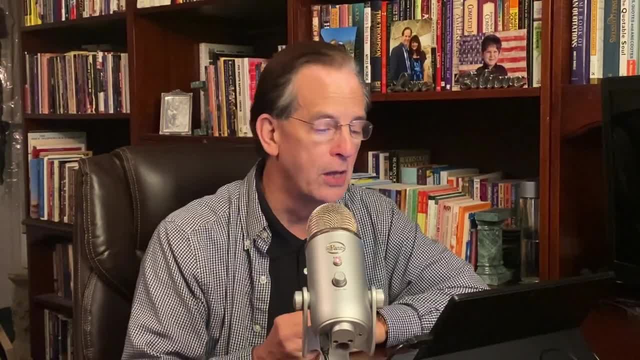 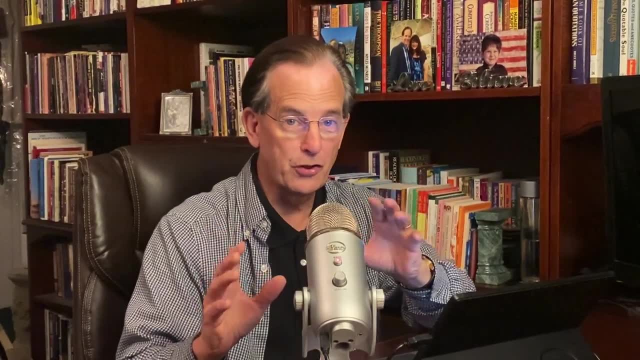 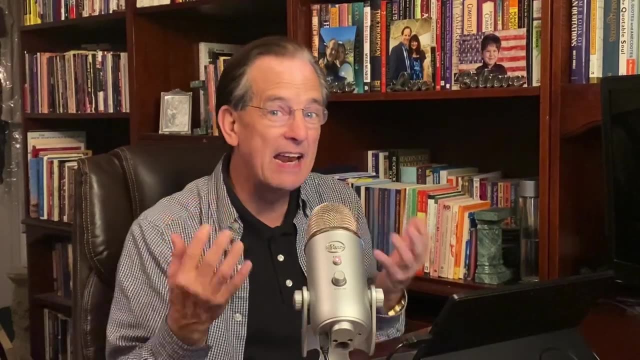 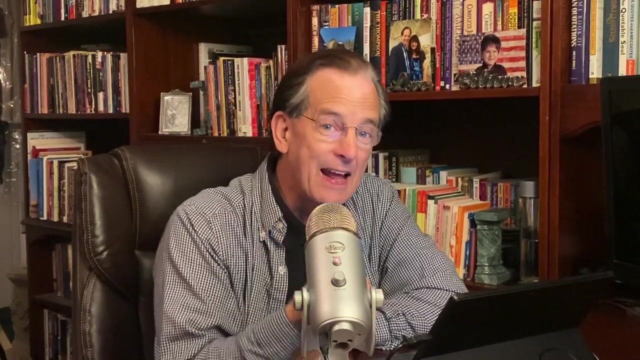 for As we practice the posture, we put our focus on the energy and the essence of the deity- And here's the disturbing part to me- And we look to embody their qualities. In other words, it is an invocation to various gods and goddesses to manifest themselves in the life. 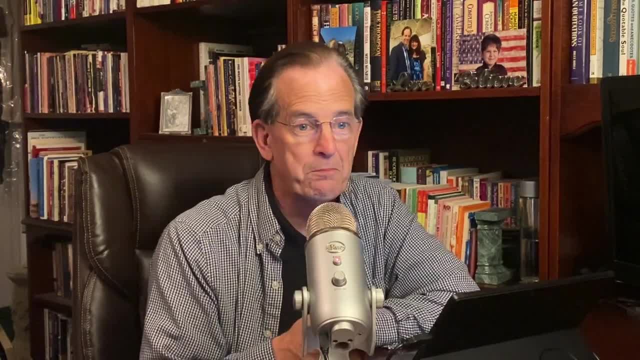 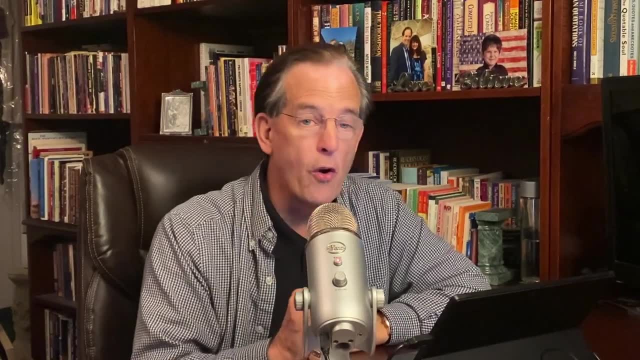 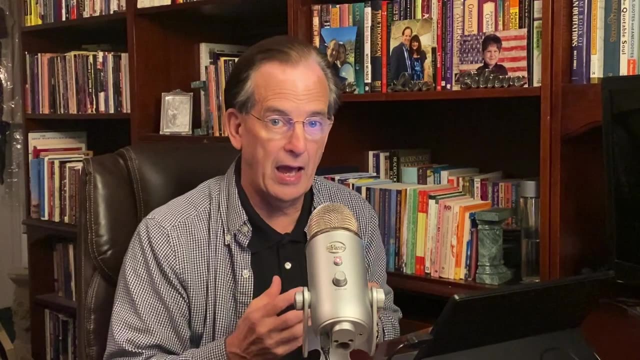 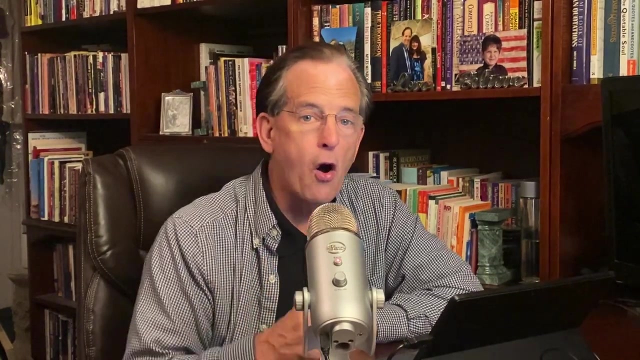 in the heart of the yoga practitioner. Now this is going to be a little challenging to communicate on the audio aspect of the podcast because I'm going to have to describe each one of the postures as I share with you the Hindu deity that particular posture is dedicated to. But we always simultaneously do a video podcast. 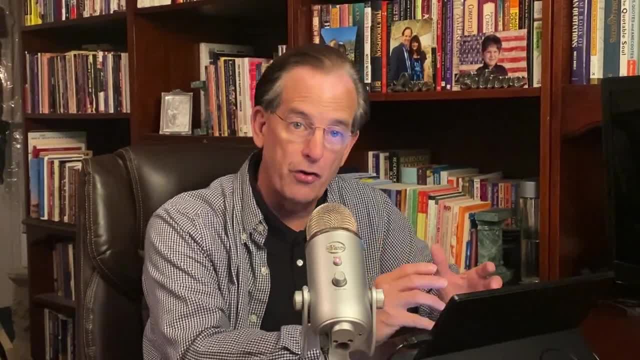 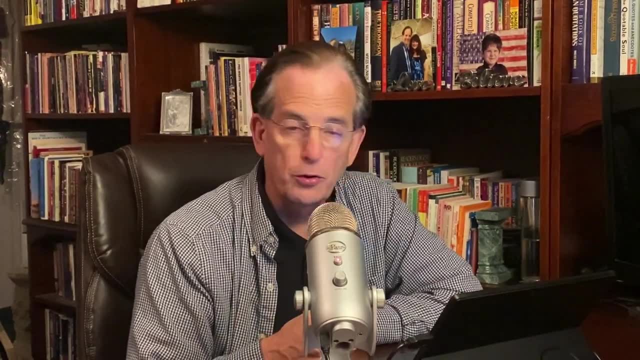 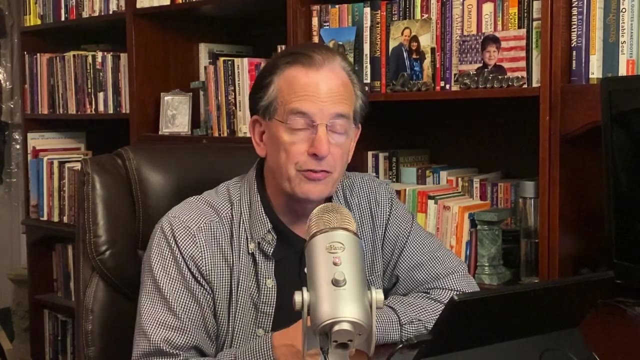 So if you'd like to see the images of the deities and also the explanation visibly of what the posture looks like, then go to our YouTube channel That's youtubecom slash- Mike Shreve Ministries, and you'll be able to not only hear this episode but see. 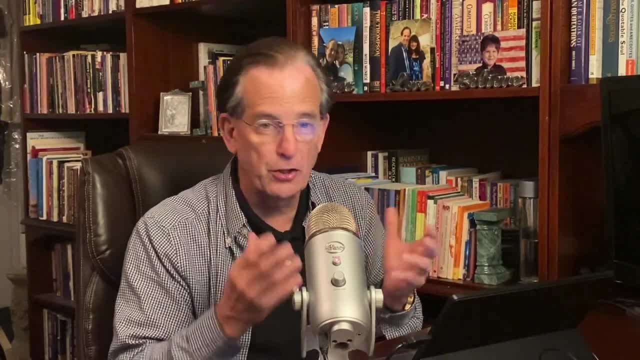 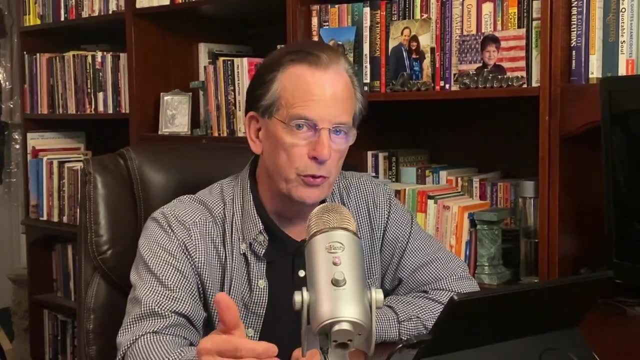 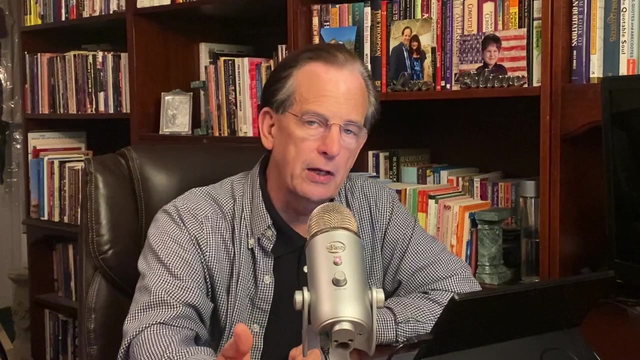 the various pictures that will help you get in your mind and get in your thinking, exactly what I'm referring to Now. most of the pictures that we will use are of children doing yoga. Why have I chosen to do that? Because recently I was contacted by a group of 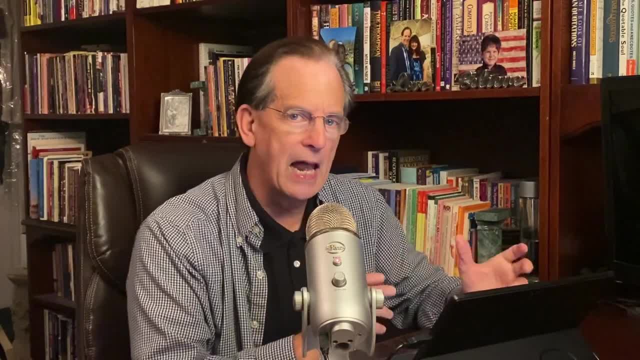 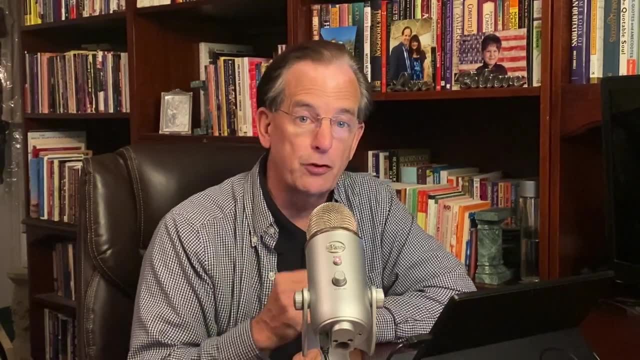 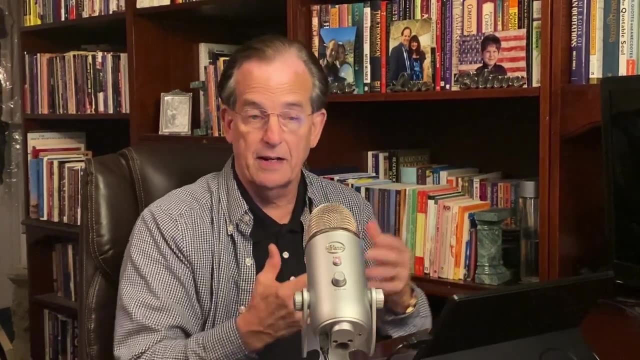 conservative and God-loving people in Alabama- leaders, influencers in that state- who were very disturbed because May of 2021, the ban against yoga being taught in the public schools was lifted. In fact, Alabama was the last of 50 states to have a ban. 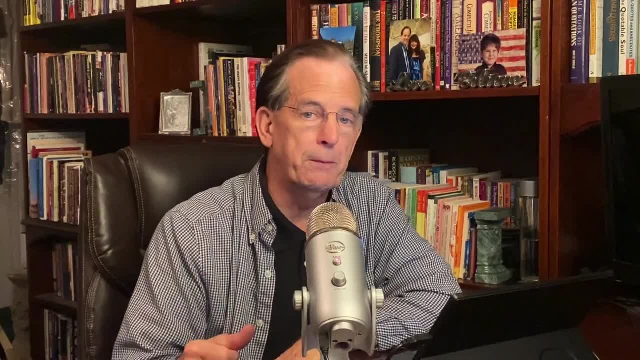 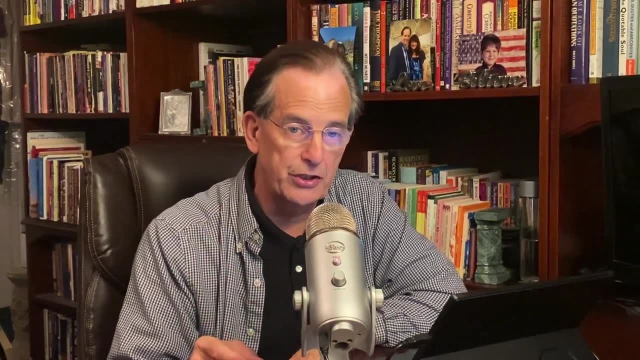 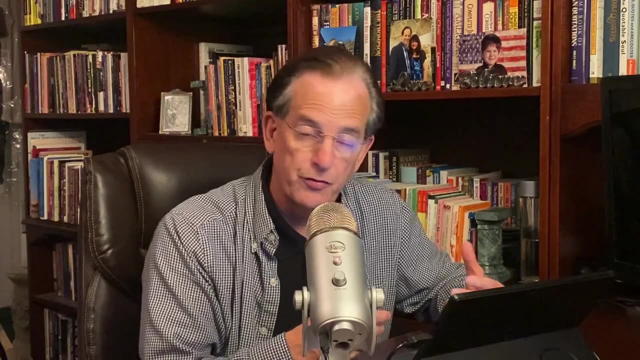 on yoga, And I mentioned to one of the people that contacted me that was a trophy in Alabama's cabinet that should not have been relinquished. But they did lift the ban and now I'm going to be working together with those individuals- very prominent individuals- to reverse that law and 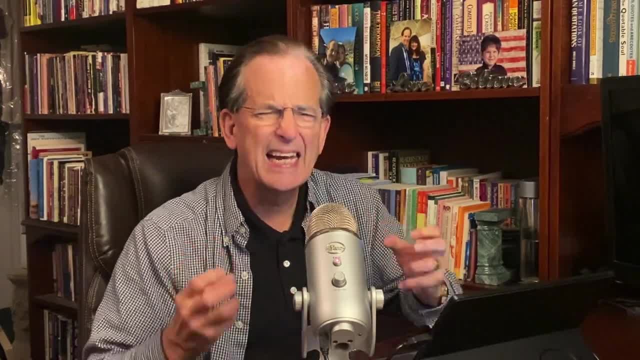 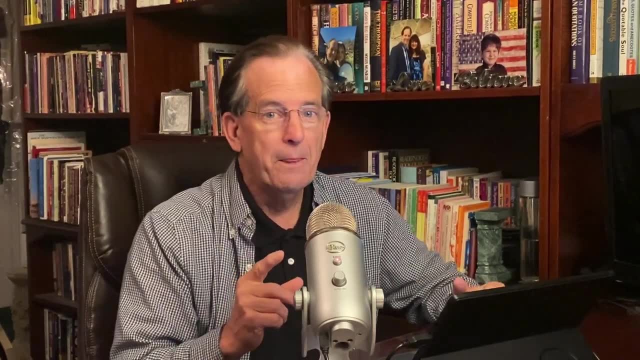 hopefully reinstate that ban, Because I cannot imagine vulnerable children doing these yoga exercises. I cannot imagine vulnerable children doing these yoga exercises. I cannot imagine vulnerable children doing these yoga exercises. I cannot imagine vulnerable children yoga postures not knowing that it is a connection to a spiritual power that is intentionally. 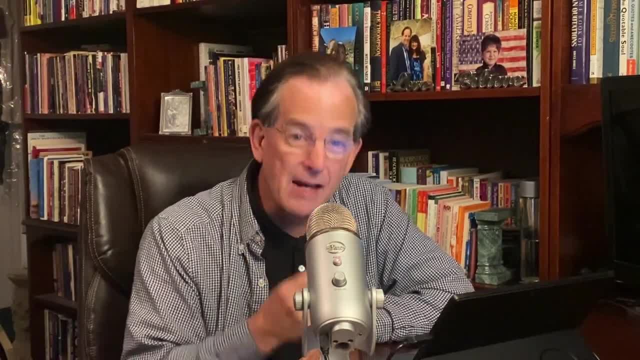 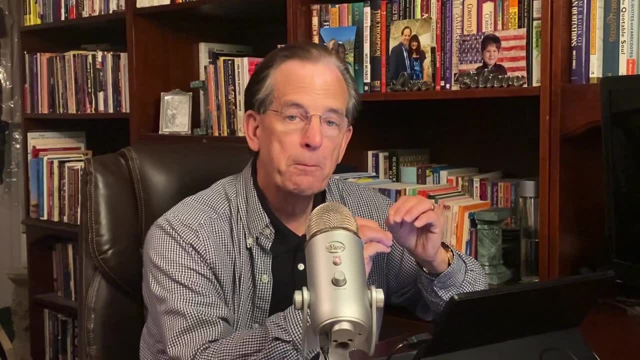 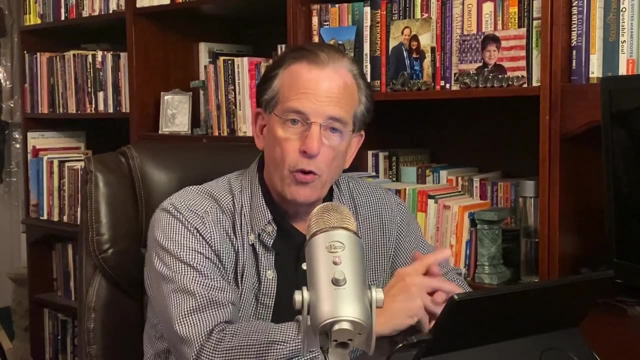 sought after by those who are serious advocates of yoga. Now, on this particular podcast, I'm going to focus on 10 positions, 10 postures that are dedicated to specific deities, And we're going to start off with the lotus position, which is the. 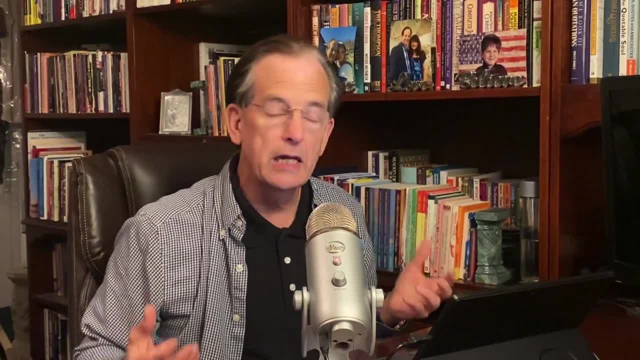 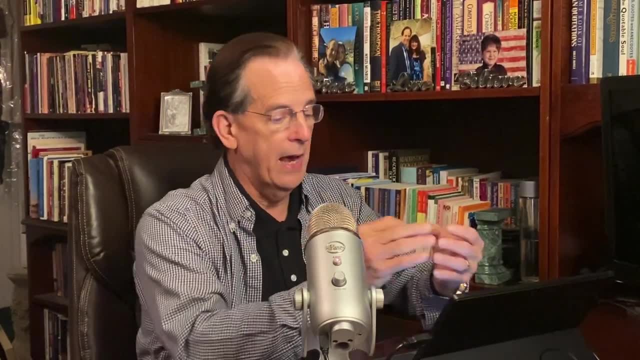 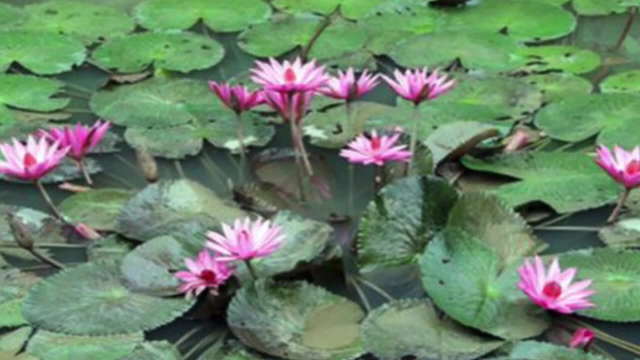 most basic posture you assume usually in a yoga class and the hand mudra. that is referred to as the jnana mudra And the posture is referred to again as the lotus position. Why? The lotus is a flower that floats on the surface of a body of water like a pond or a lake or a creek. 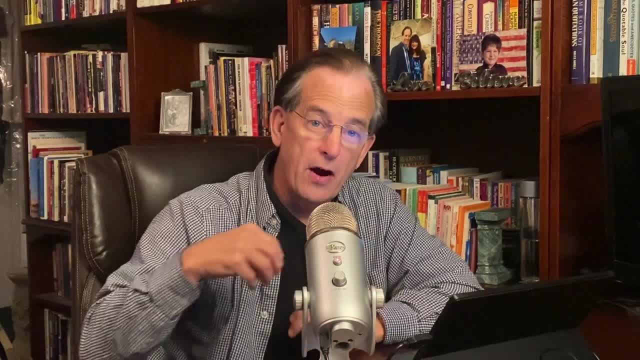 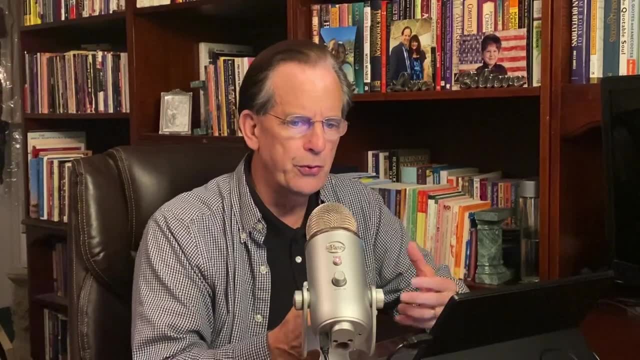 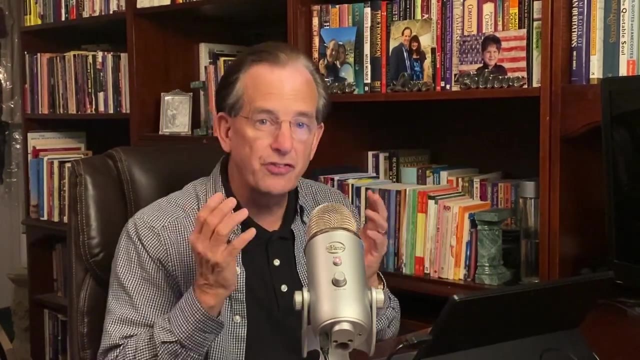 And the roots of that lotus are in the mud beneath the surface, And so it represents symbolically those who rise above the lower nature, those who rise above the sense bondage that every human being is in, being cognizant only of what we see. 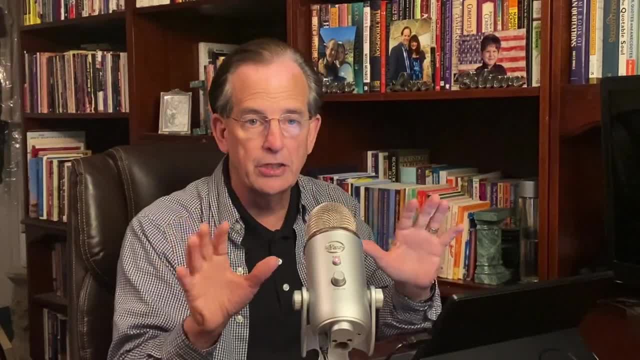 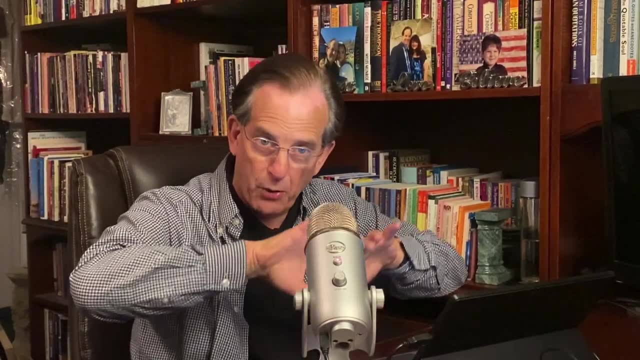 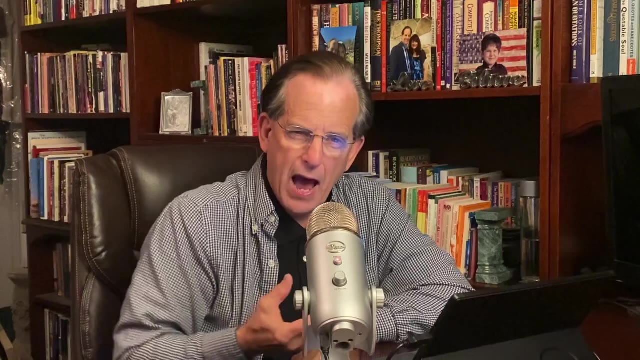 what we hear, what we smell, what we taste, what we touch, And that's like a prison of the five natural senses And most individuals never break beyond the bounds or limitations of those senses. But the lotus flower represents rising up through the limitations. 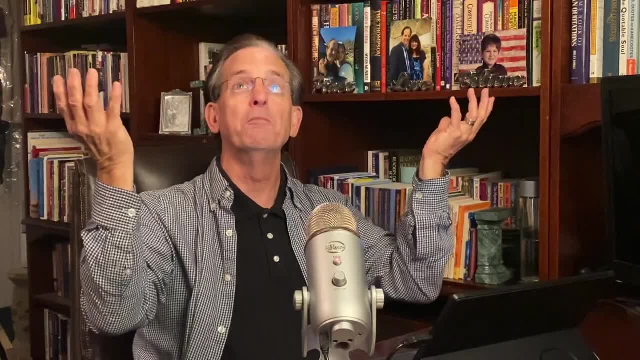 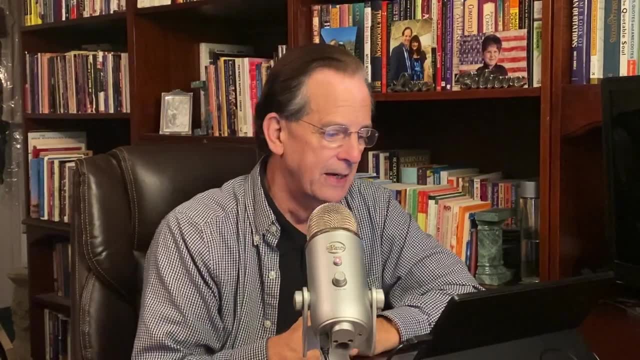 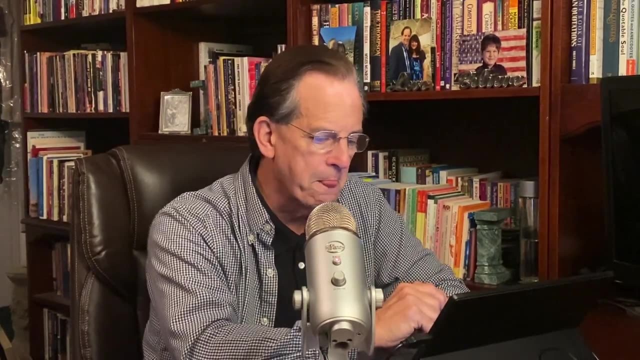 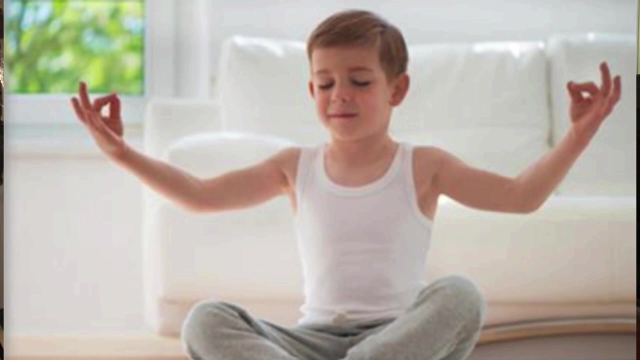 on most human beings to blossom above the constraints, the boundaries of human consciousness. That's why it's considered a sacred symbol, a sacred flower, in most Eastern religions. Now, what about the gyan mudra, which is the position of the forefinger touching the thumb and the other three fingers extended? 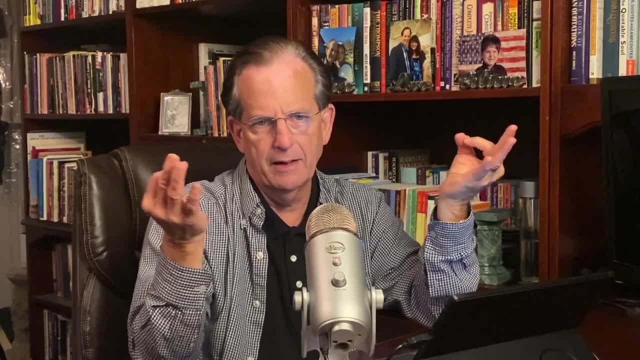 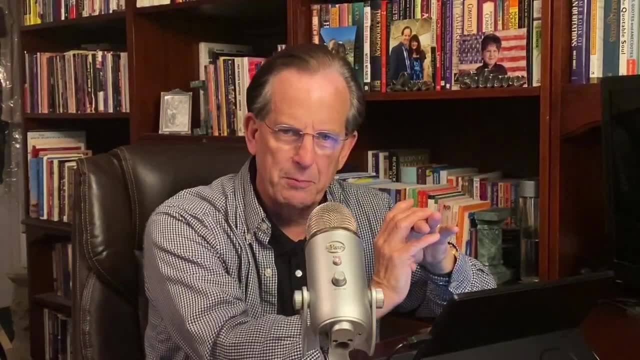 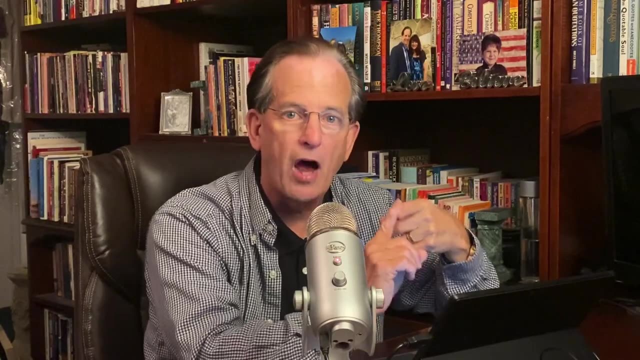 outright. What harm could there be in that? Of course it's taught that that helps the energy to circle through your body, But there's a spiritual symbolism attached to it. The forefinger represents the individual soul, which is referred to in Hinduism as Atman. The thumb represents the 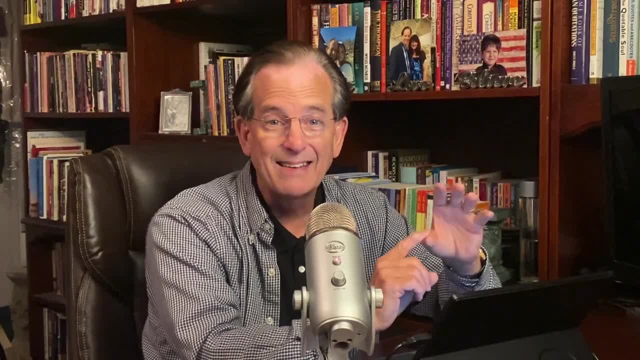 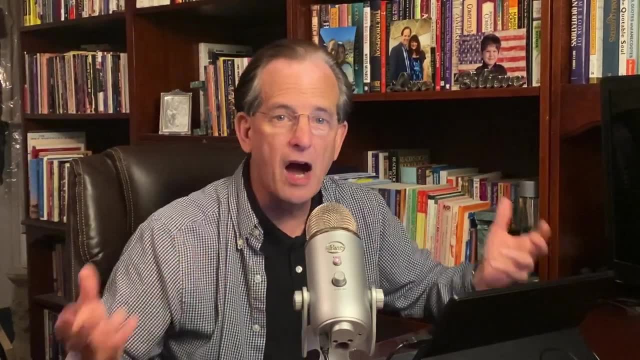 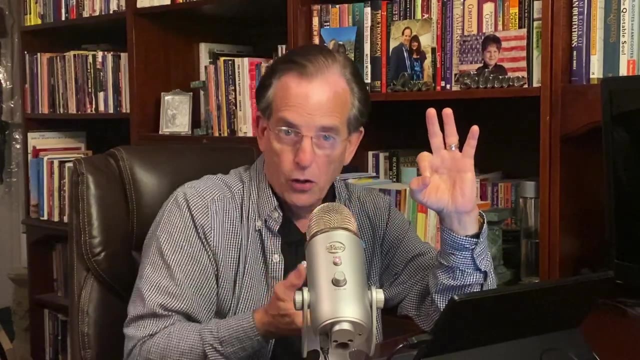 oversoul, or the ultimate realization of the body through the Prayer of the Lord. So it represents reality in Hinduism referred to as Brahman, which is a cosmic force, a level of consciousness, not a personal God. And when someone assumes the lotus position and then curls their forefingers, 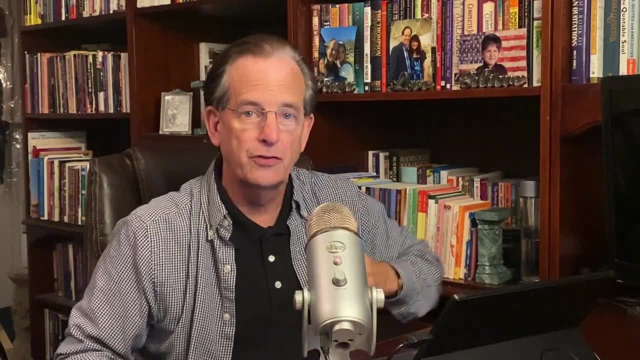 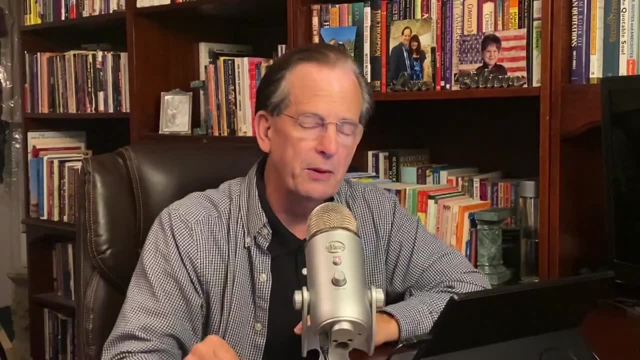 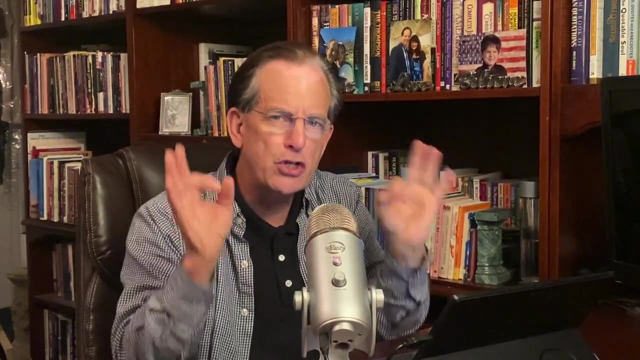 around to touch their thumbs, and usually they rest their hands on their knees. the picture is of a child raising his hands upward, but still assuming that mudra, It is a prayerful statement that the individual soul will come into union with Brahman with this ultimate reality that 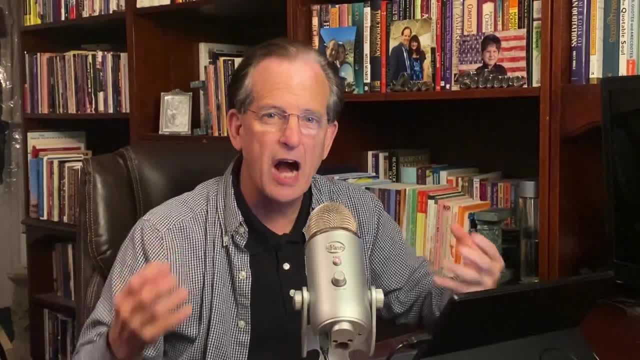 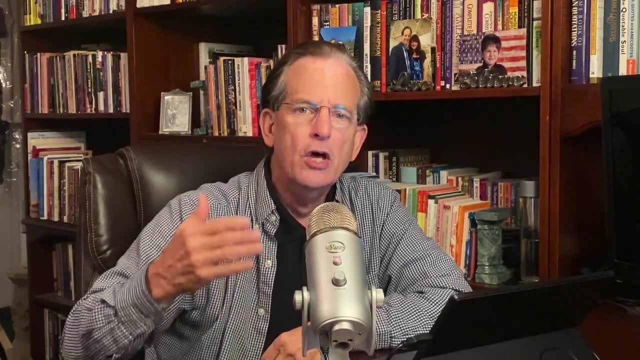 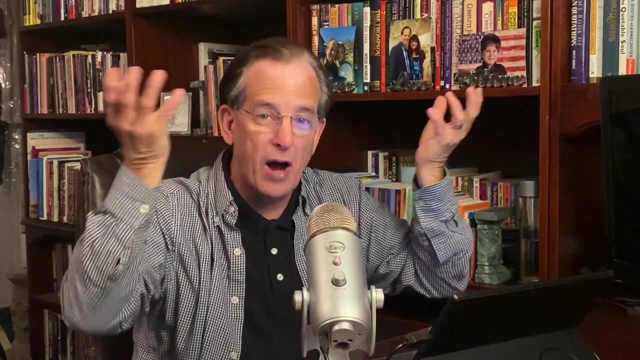 is envisioned as an impersonal life force, a cosmic level of consciousness. Well, that is not the true God and that is an invocation, therefore, to a false God to take you over, To manifest within you and to bring you up to a higher level of consciousness, like the lotus. 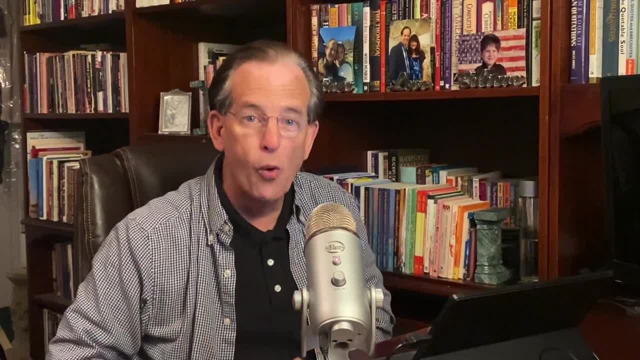 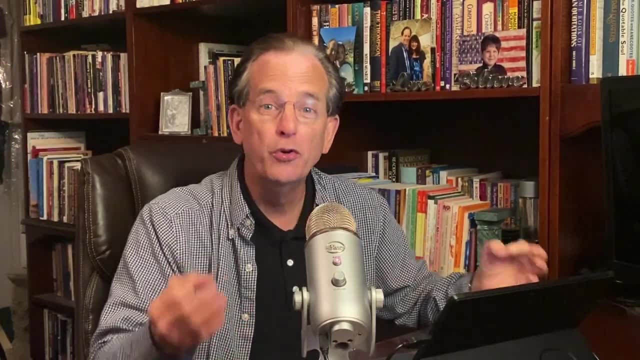 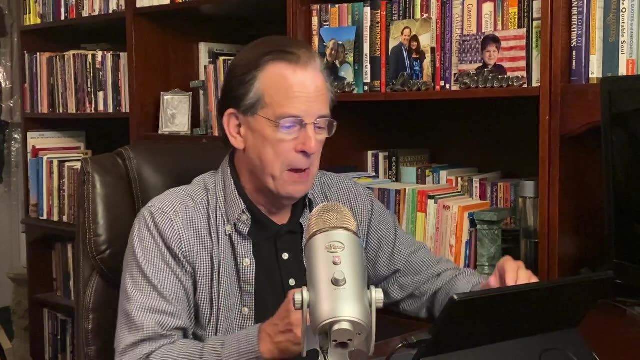 flower breaking out of the limitations of the lower nature. Well, that may not be what you intend for it to mean. when you assume that position in a yoga class, You may think you're just getting ready for an exercise session, but what you're doing is very symbolic spiritually. 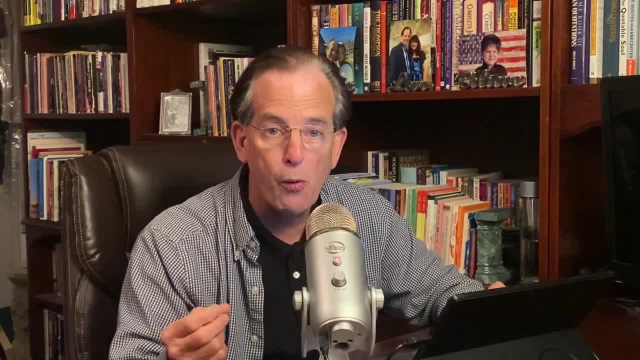 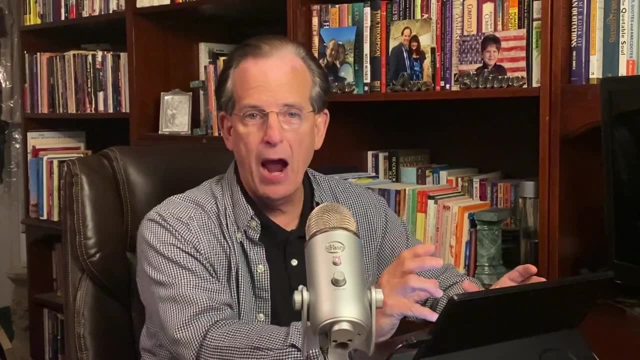 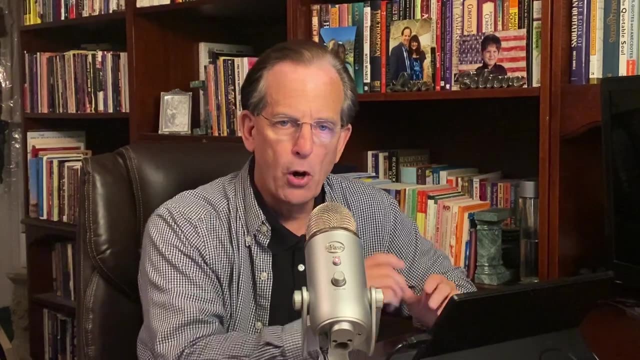 and very, very much an attraction to powers that are supernatural, that are not the power of the Holy Spirit. It's a different power altogether that you access during the yoga sessions. Now, the second pose that we're going to focus on is the tree pose, And for the sake of those, 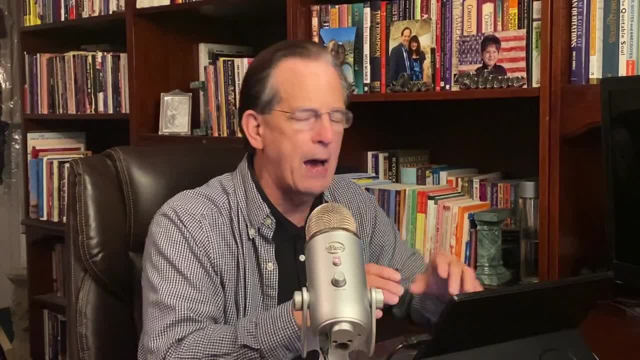 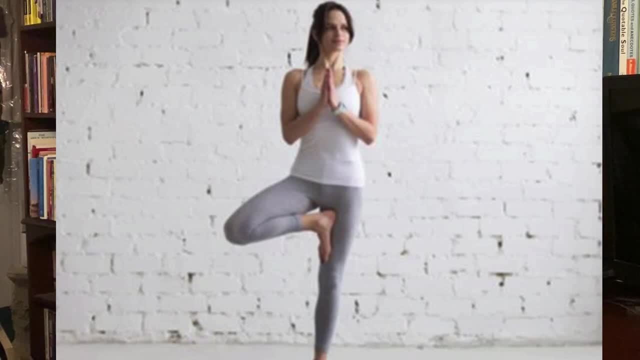 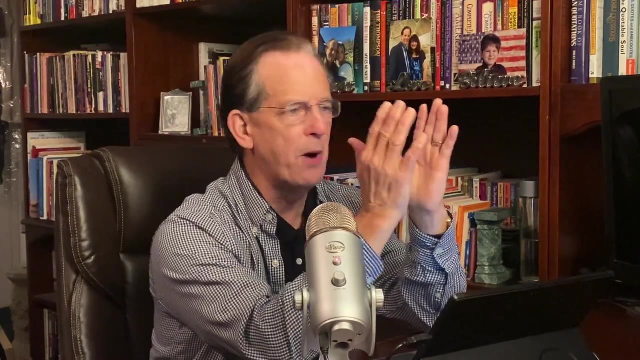 that are listening to this on the audio podcast. I'll describe what it looks like. You stand on one foot and the other leg is bent at the knee and the foot is placed next to the opposite knee And then the hands are lifted in a prayerful palm-to-palm position, And that's referred to again as the 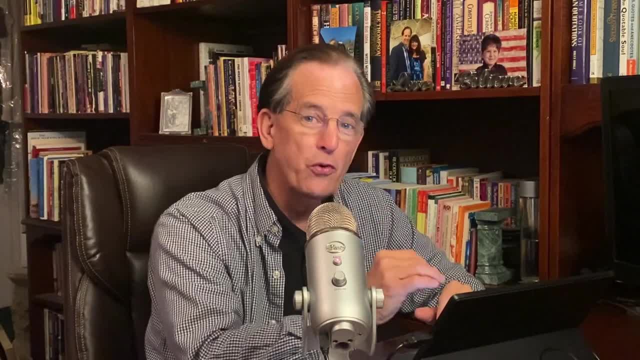 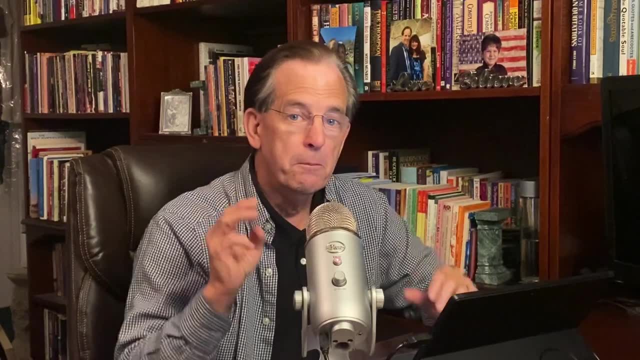 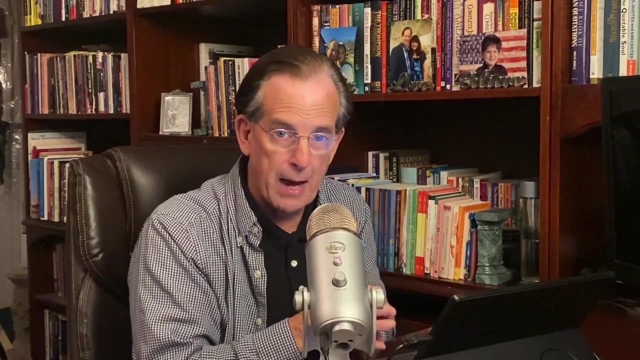 tree pose. Now that particular pose is dedicated to the Hindu deity named Vishnu, And Vishnu is one of the three most revered deities. It's called the Hindu triad. It's not the same as the trinity of the Bible- not at all, But there is a similar kind of approach where there are 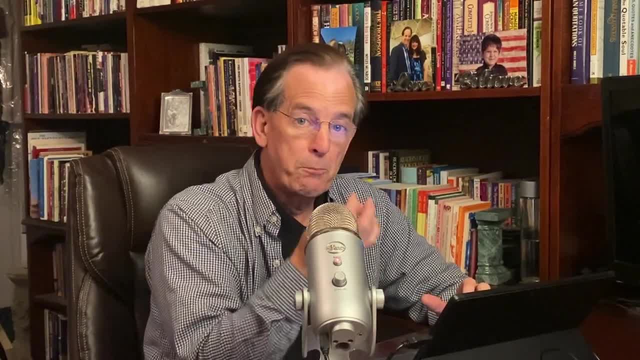 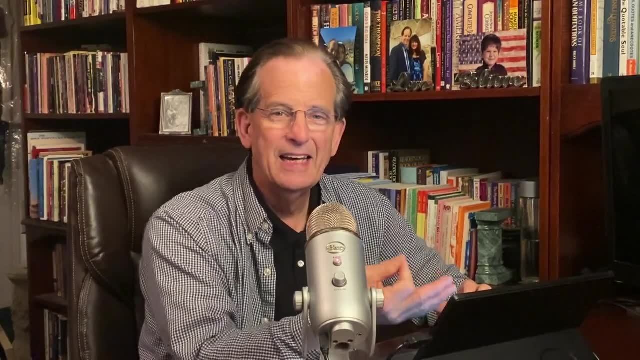 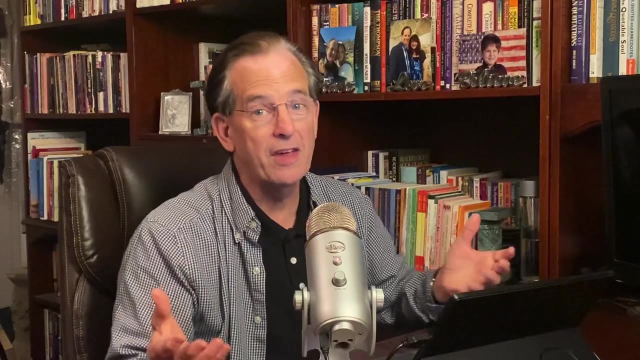 three revered deities Now: Brahma is the creator god, Vishnu is the preserver god and Shiva is the destroyer god. And we're going to get to Shiva next, But they're part of a pantheon once again. 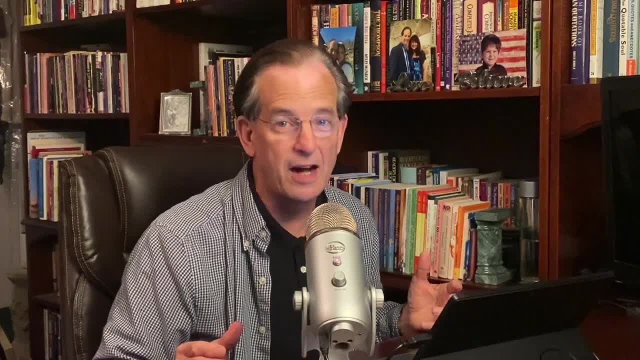 of 330 million gods and gods, And they're part of a pantheon once again of 330 million gods and gods, And they're part of a pantheon once again of 330 million gods and gods, And they're part of a. 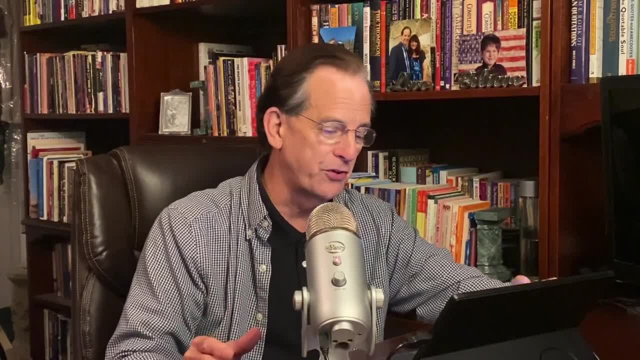 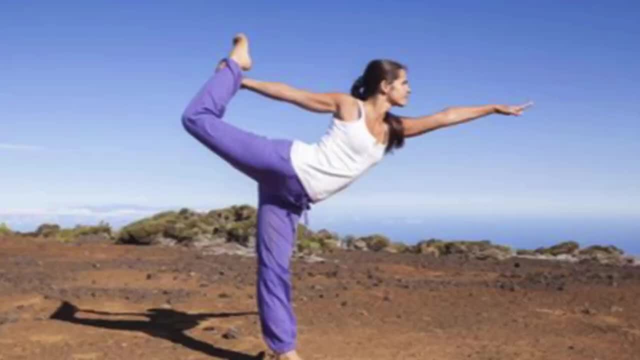 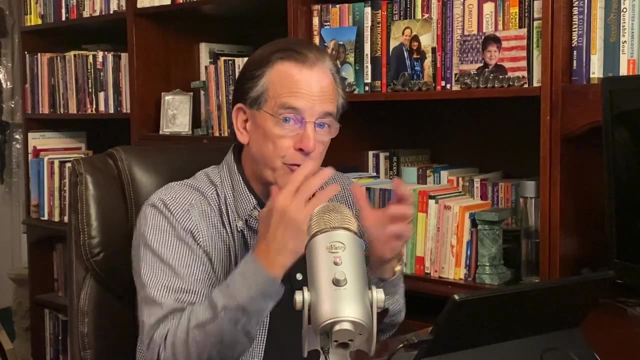 which is the traditional number, certainly not an exact number. Now, number three is the dancer pose, And the dancer pose is dedicated to Shiva, the destroyer god, who is the source of the destruction and rebirth of the universe during cycle after cycle. 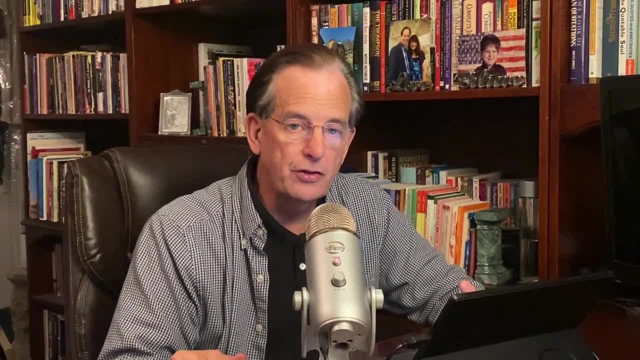 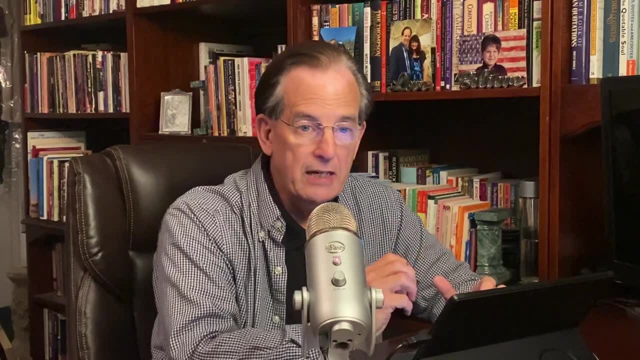 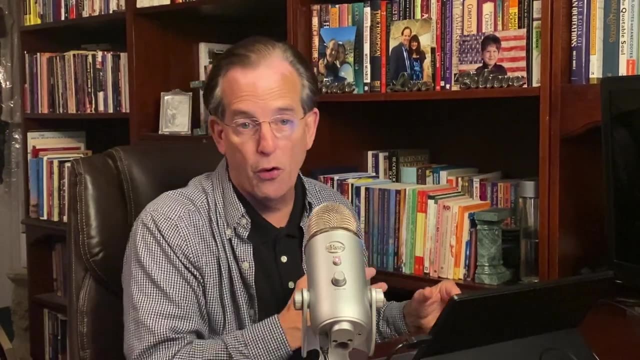 endless cycles, according to Hindu teaching, of the universe being dissolved and then reappearing, And Shiva is the one who affects that. And also Shiva is the source of the death and rebirth of the soul in various reincarnations. 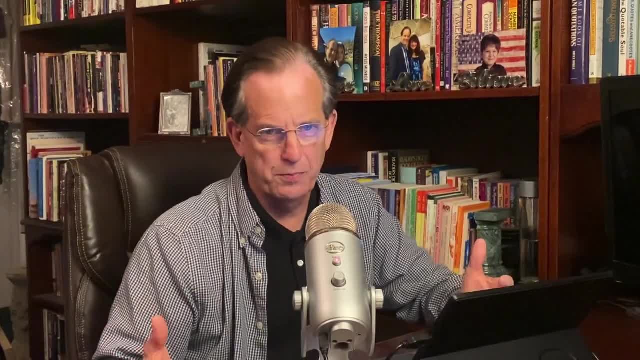 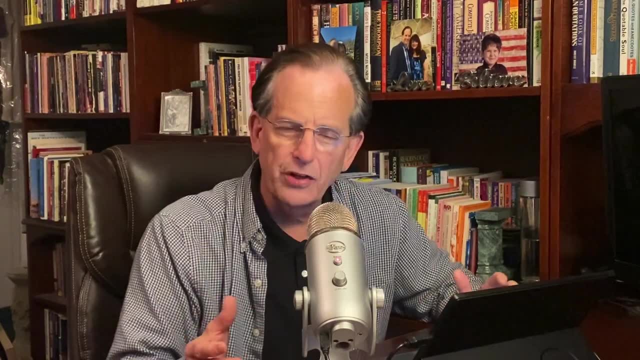 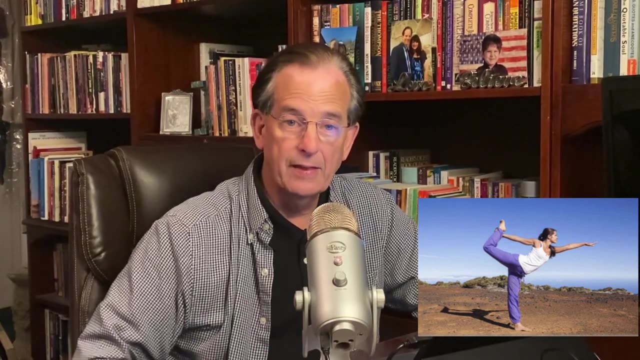 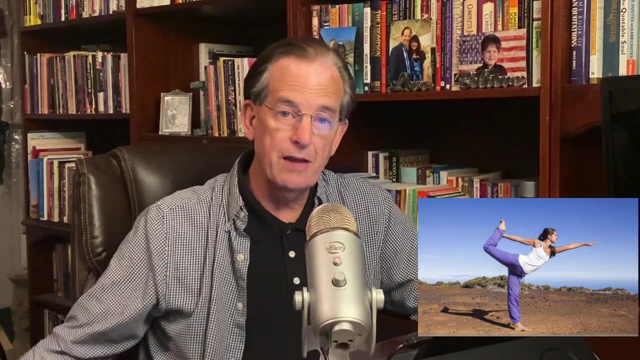 And that's the cosmic dance, so to speak, And so the dancer pose is dedicated to the one who affects that. Now, what does it look like? The person assuming that pose stands on one leg again and then lifts the other leg behind him or her and then grabs the foot and lifts the leg up. 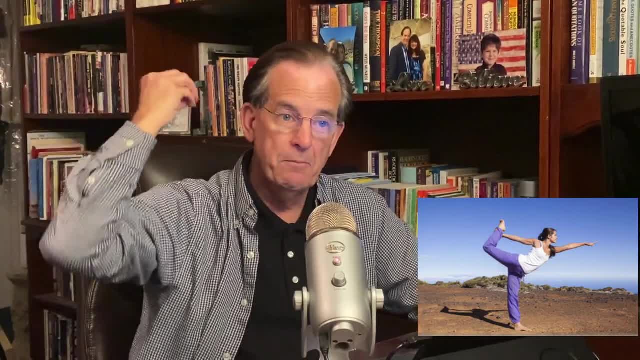 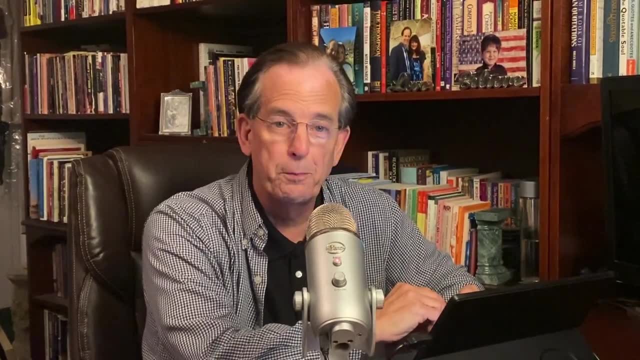 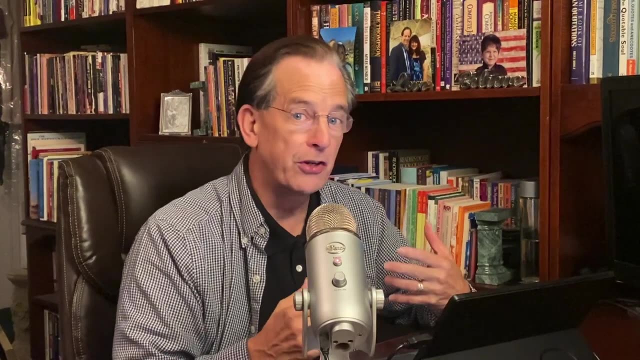 in a circular fashion behind the head and then tries to balance in that pose. And again it looks like just a harmless physical position, but it's a spiritual connection to the deity of destruction. Now in the Bible, the destroyer is not a deity. 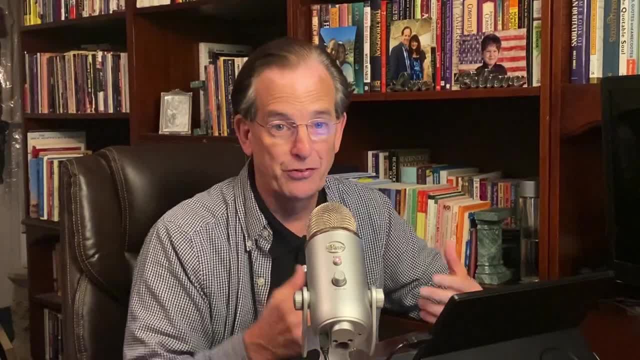 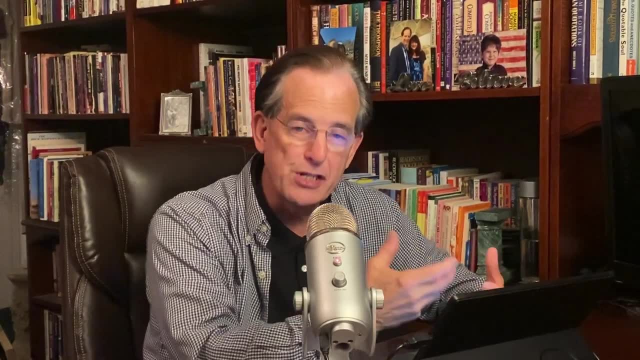 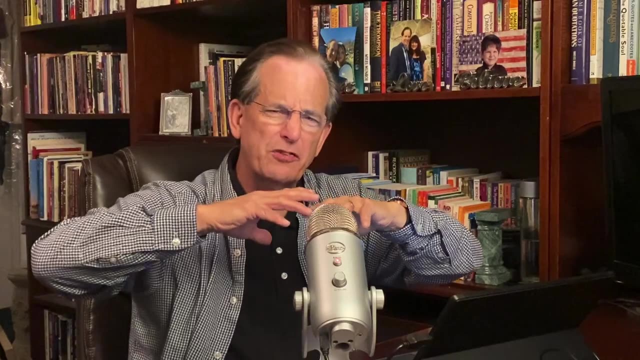 unless you were to refer to him as the god of this world, as Jesus referred to him, Certainly not a god to be worshipped, but an entity of great spiritual power. Satan is the god of this world in the sense that his spirit controls the nature of this planet and has infiltrated societies and 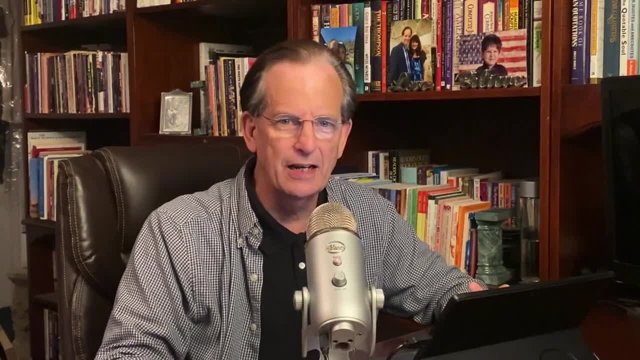 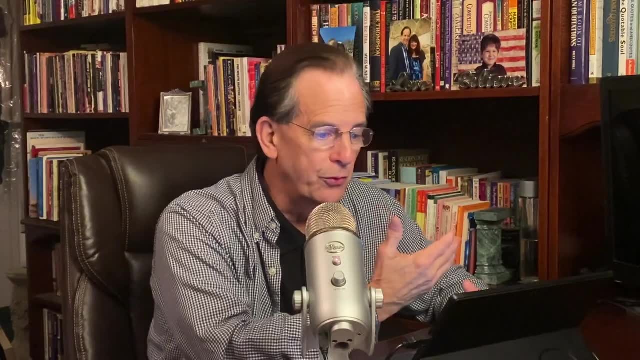 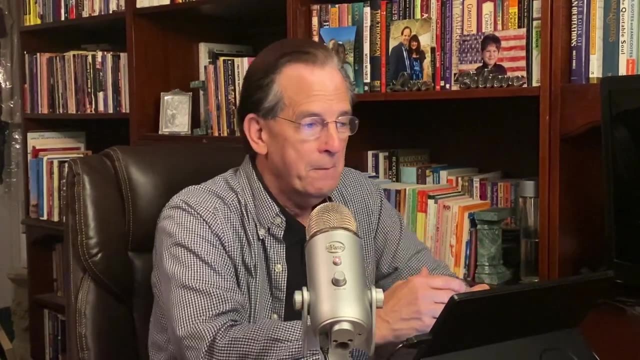 cultures and has contaminated the human race. The spirit that works in this world, the spirit that works in the children of disobedience, is traced right back to Satan himself. He is the destroyer. In fact, that's very much what the name Satan really represents. He's the hater, He's the 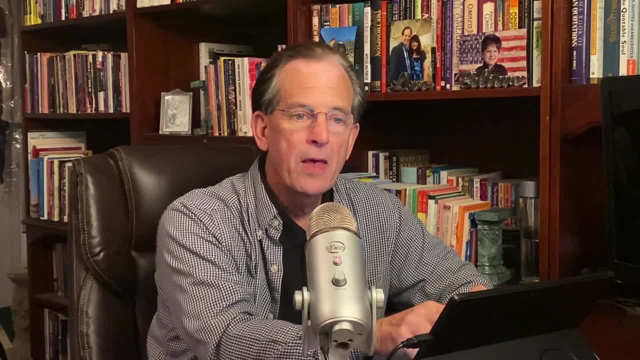 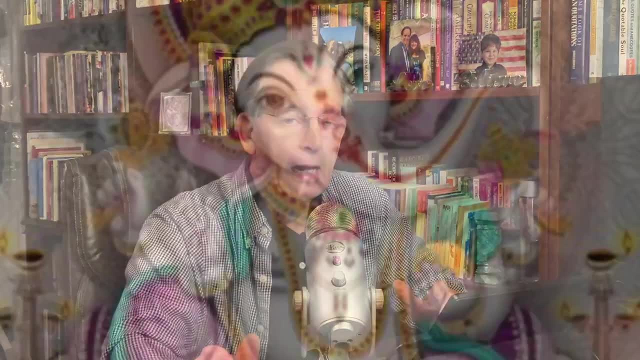 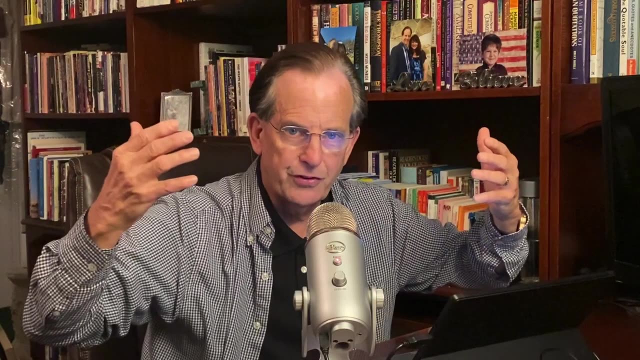 destroyer of the human race. Now, number four is the warrior. number two pose That is dedicated to a god named Ganesha, And Ganesha is the destroyer of the human race. And Ganesha is the half-human and half-elephant. From the shoulders up, it's the head of an elephant From the 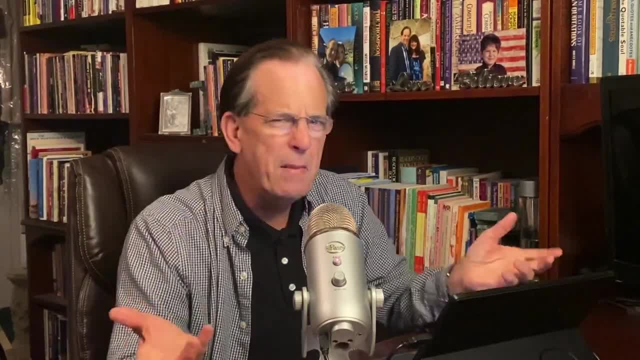 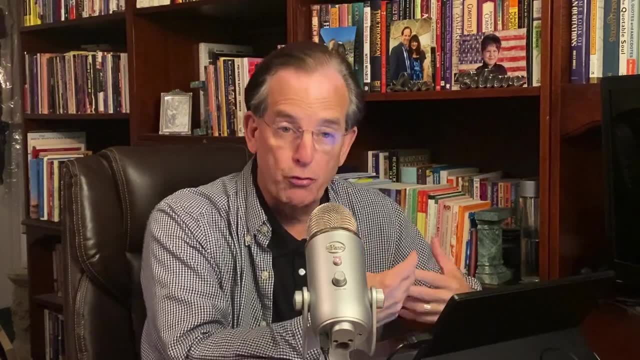 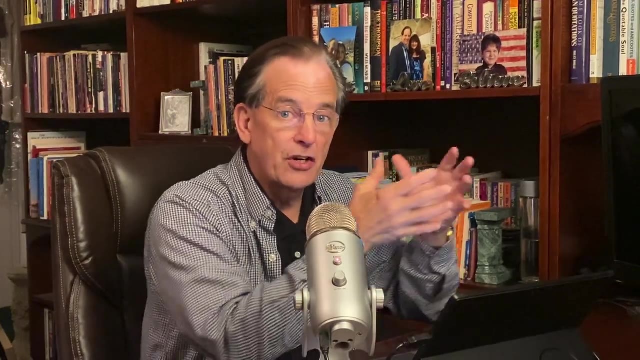 shoulders down. it's the body of a human, And there's a myth about how that took place. Actually, this was a deity created by Parvati, a female goddess who wanted this deity to guard her while she was bathing in her home, And her consort, her husband. 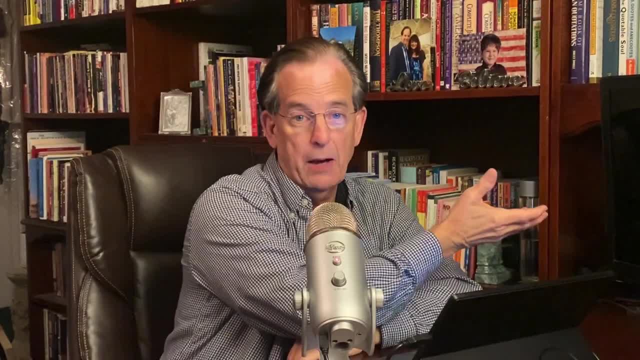 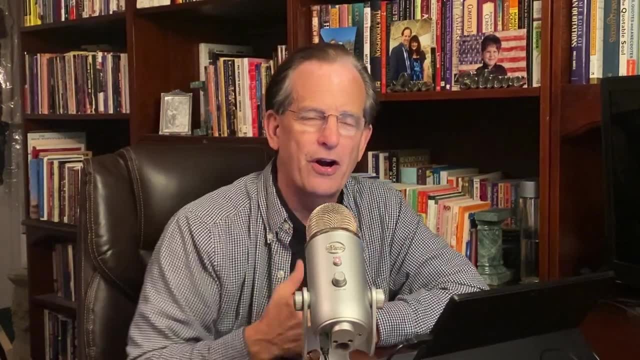 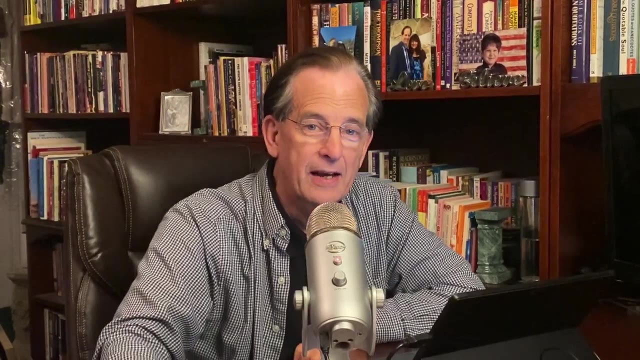 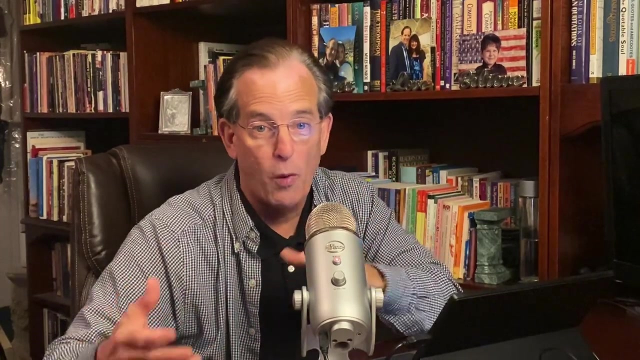 so to speak. Shiva was gone, And when he came back, this created being that Parvati had created in order to guard her home refused him entrance, And so Shiva lopped his head off, And when he found out that, actually, that entity was not an enemy, but one who was guarding his wife or his 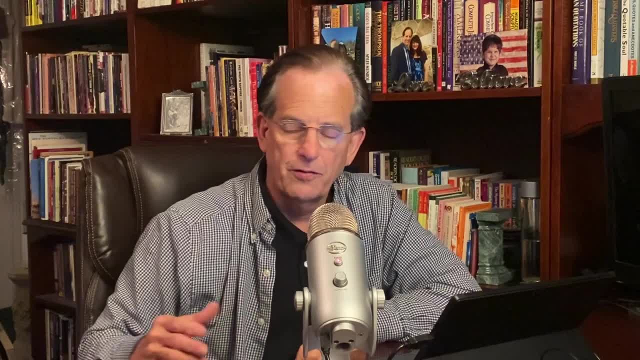 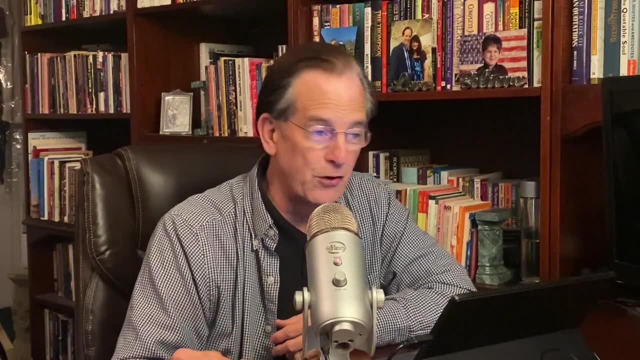 consort. then he sent some of his servants down to the earth, And the first thing that they did was to cut off the head of the first living thing they came to, And, unfortunately, the first thing encountered was an elephant, And so they brought the head. 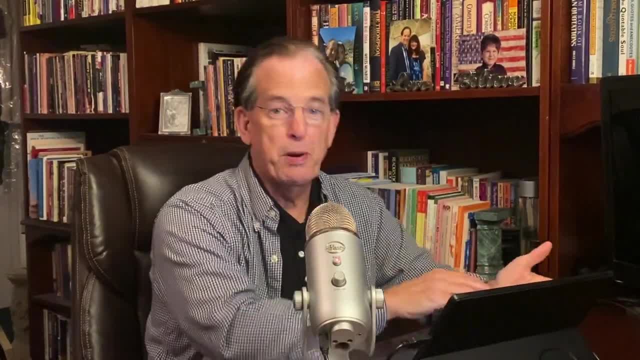 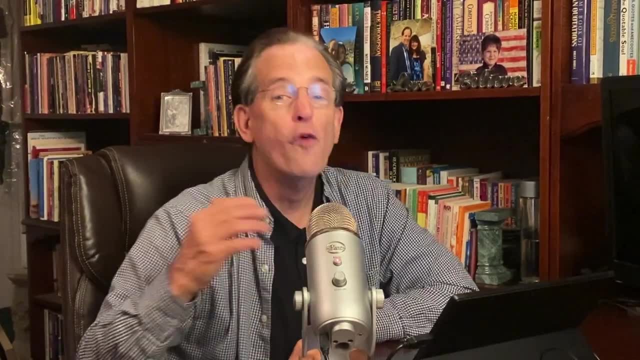 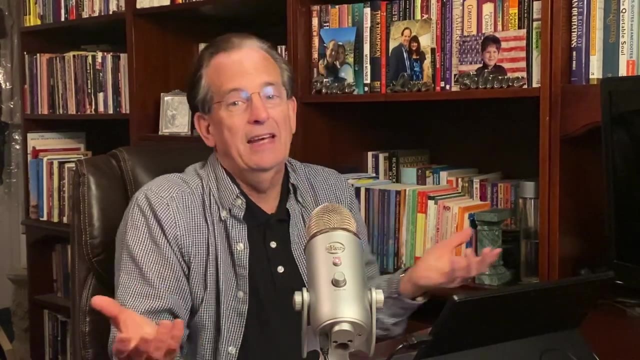 of the elephant back to the celestial world. It was placed on this entity's body And thus the deity that is an overcomer of obstacles, was brought into being, And that deity is named Ganesha, And you see that deity depicted many times. Well, when you assume that Ganesha is, 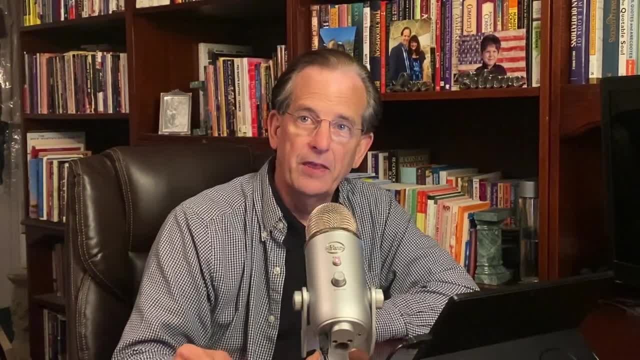 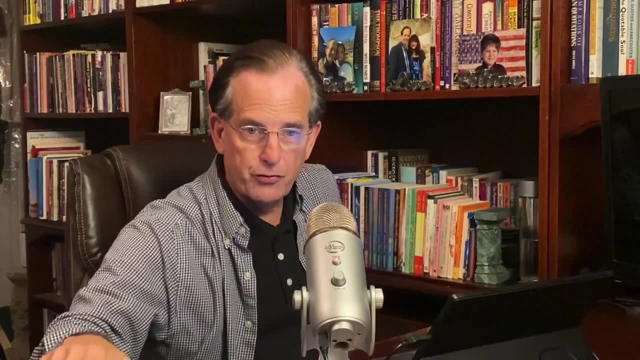 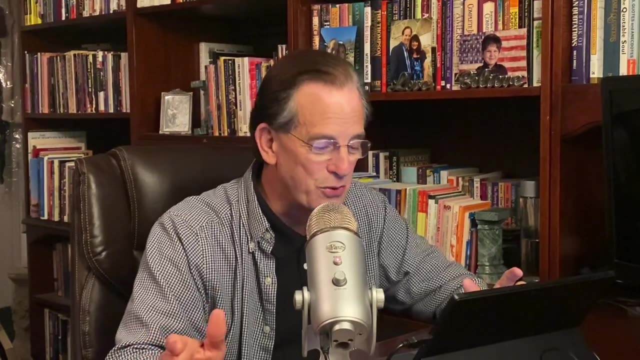 the warrior pose, which is a pose where the one arm is stretched out to the front, the other arm is stretched out to the back and both legs are stretched apart, as if a person is about to lunge forward. But that's a connection to a false god. The next pose is the splits pose. 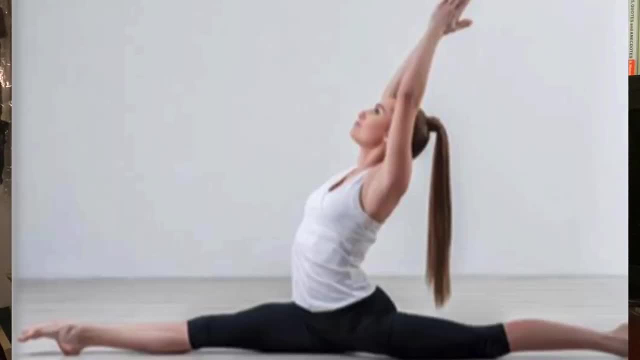 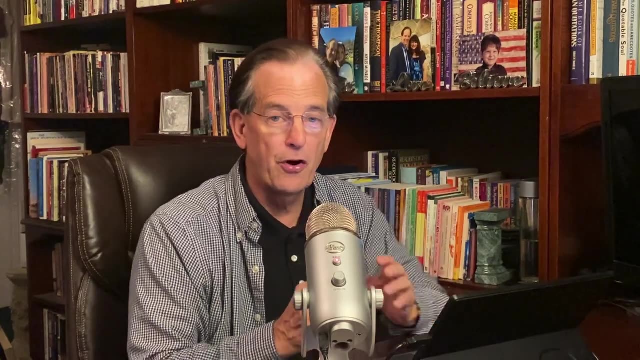 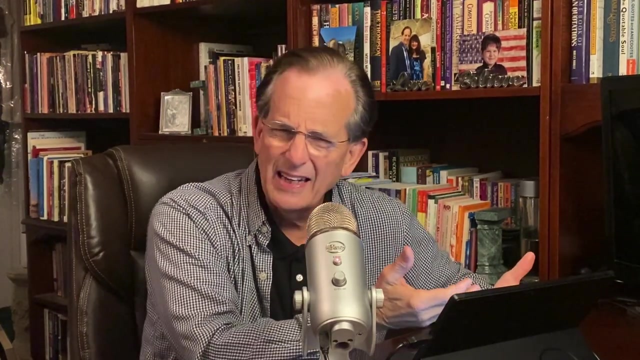 And that's, of course, where the legs split to opposite extremes, But usually the one participating in that posture lifts his or her hands above their heads in that prayerful position of palm to palm. Now, who is that dedicated to? Or is that just? 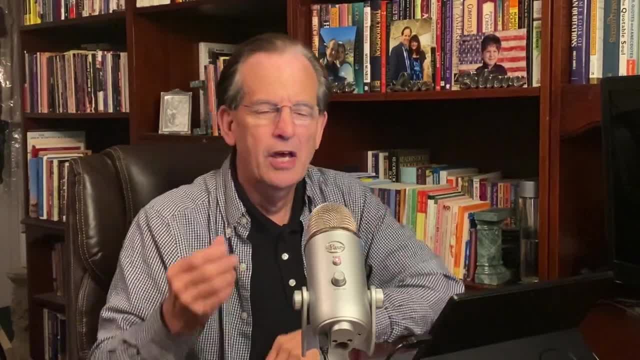 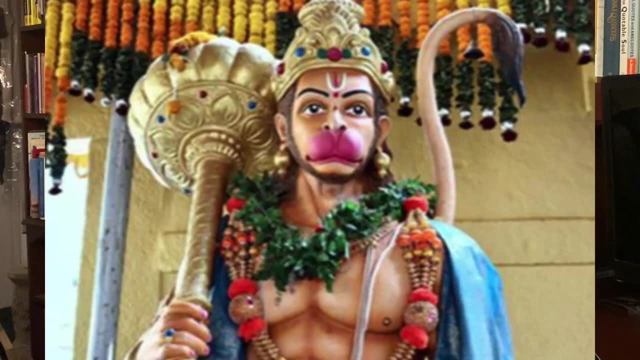 a split like you would do in a gymnastics class. No, that particular pose is dedicated to the god Hanuman, which is a god who has the appearance of a monkey and a man and is the blending of an animal, And so Ganesha is the one who is dedicated to the 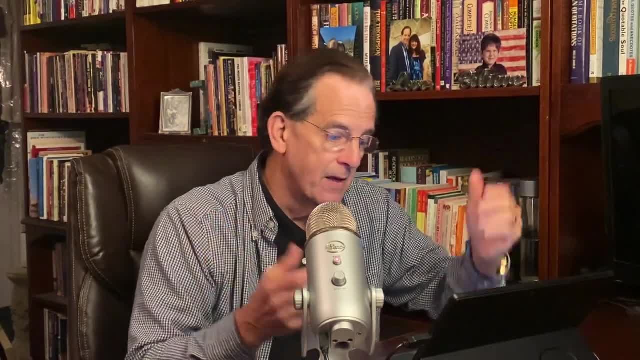 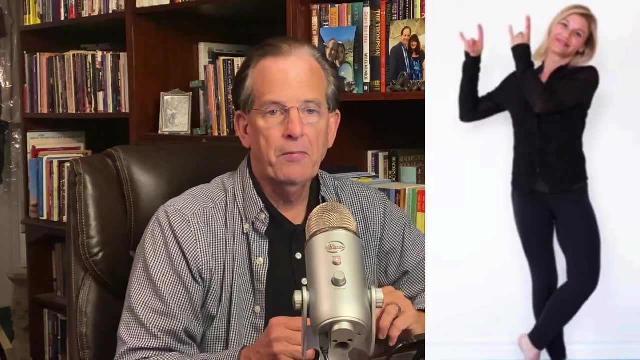 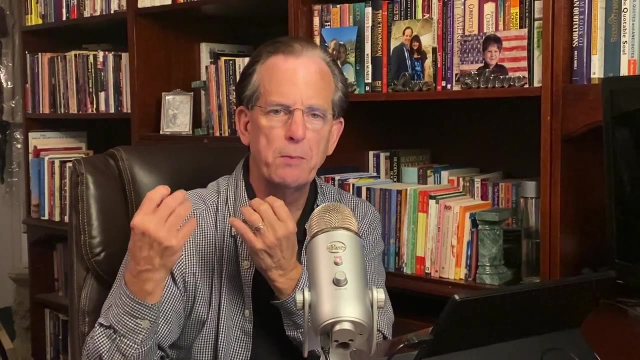 animal and a human appearance. The standing pose is the next one, And the standing pose requires a mudra as well, And that mudra is what appears to be the hand position of someone playing the flute, which is something assigned to Krishna. Now, Krishna is one of the most. 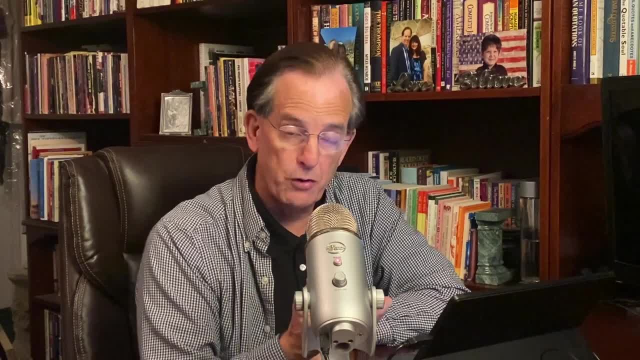 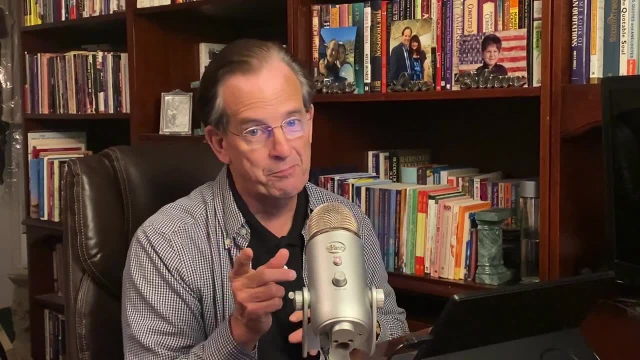 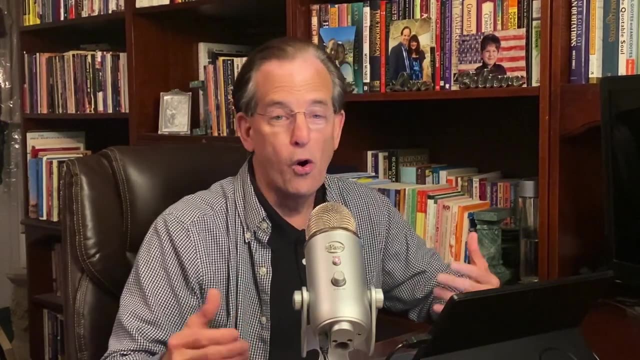 revered Hindu deities. Many people are Krishna devotees, and some who are devoted to Krishna say that Krishna is the ultimate reality, not Brahman, And so there is disagreement within the ranks of those who embrace Hinduism over who or what constitutes ultimate reality. 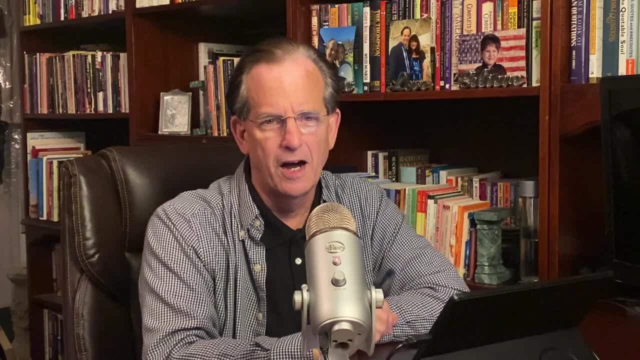 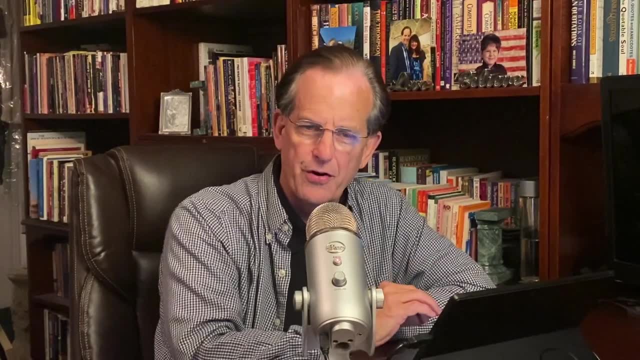 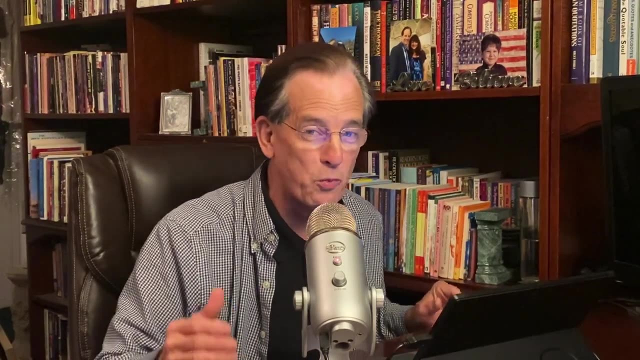 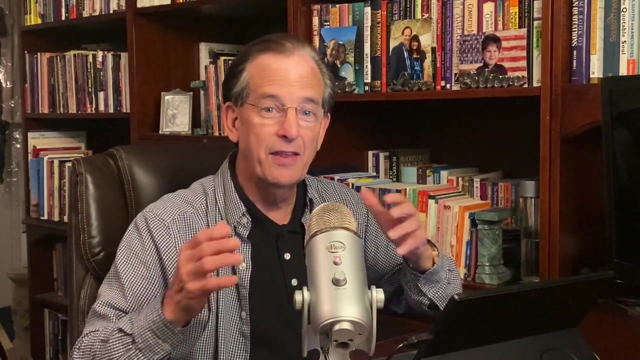 But according to the myths associated with that, god Krishna had 16,108 wives when he was on the earth And by each one of those wives he had 10 children and he separated himself into 16,108 forms so he could live in a palace with each one of those wives and those children. 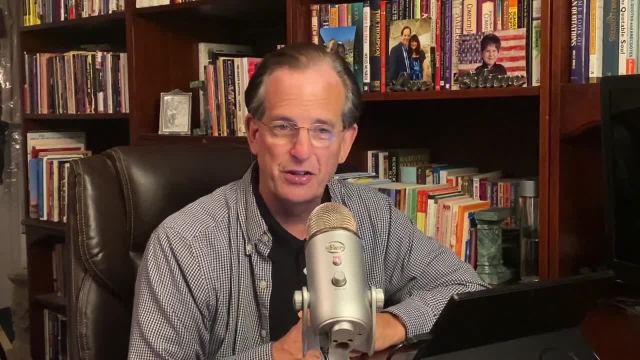 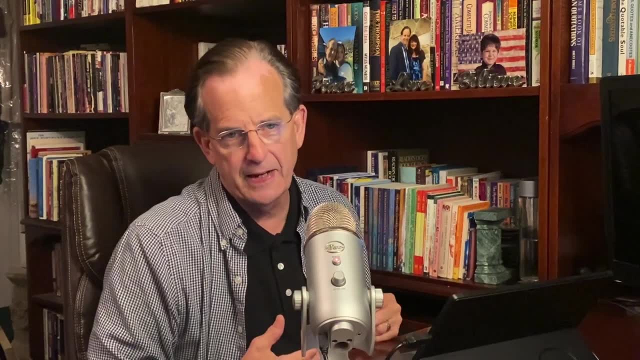 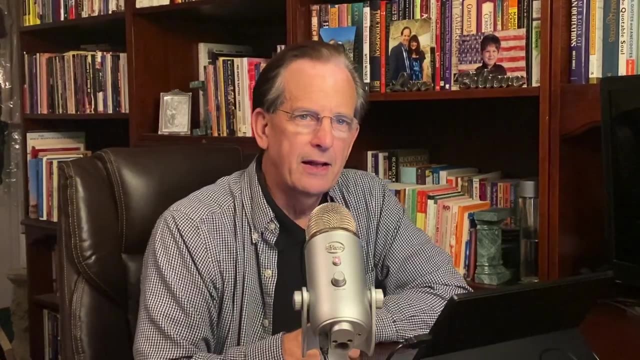 Now does that sound like a believable myth to you? And yet, when the standing pose is assumed, which is a very simple pose- crossing the feet, standing erect and then holding the hands in a mudra form- that is a connection to a false god. And so, when the standing pose is assumed, 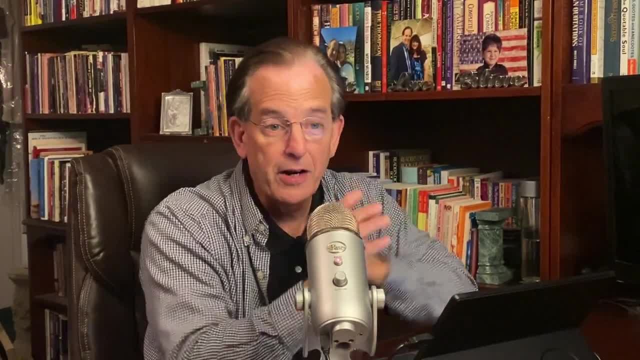 which is a very simple pose: crossing the feet, standing erect and then holding the hands in a certain mudra form. that is a connection to a false god. The next pose is a very disturbing one When you see the goddess it is dedicated to. it's actually. 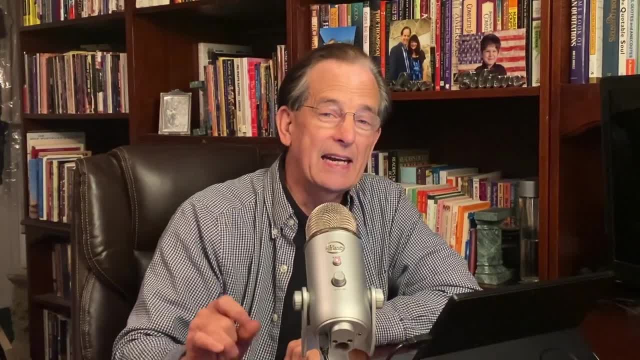 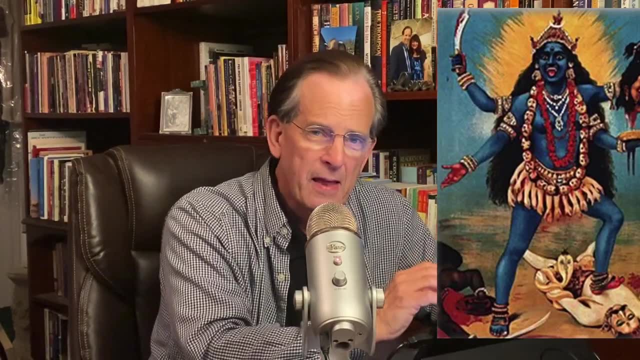 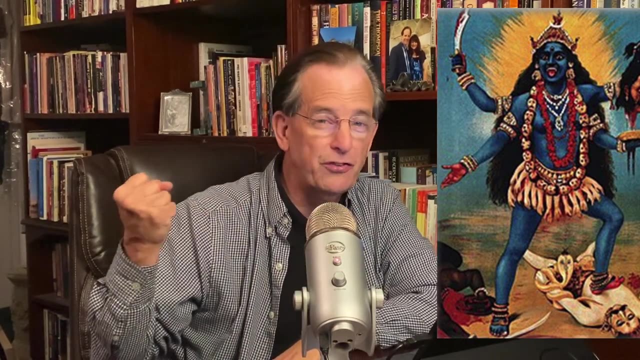 called the goddess pose, And it is a worshipful offering to the goddess named Kali. Now, Kali is depicted as a very vicious being. In fact, in the picture that I provide, she has a bloody sword in one hand, a decapitated head and a sword in the other, And she has a bloody sword in one hand. 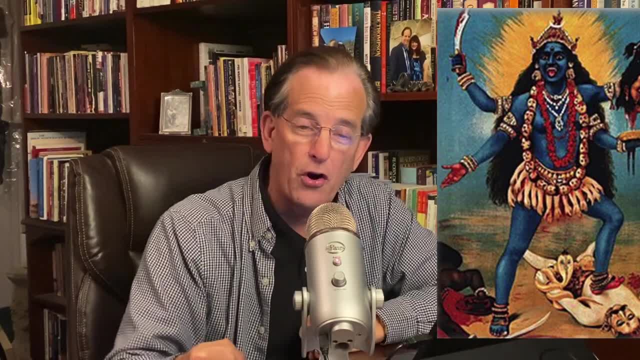 a decapitated head and a sword in the other. And she has a bloody sword in one hand, a decapitated head in the other. She is standing with one foot on the god Shiva And there is a necklace of skulls. 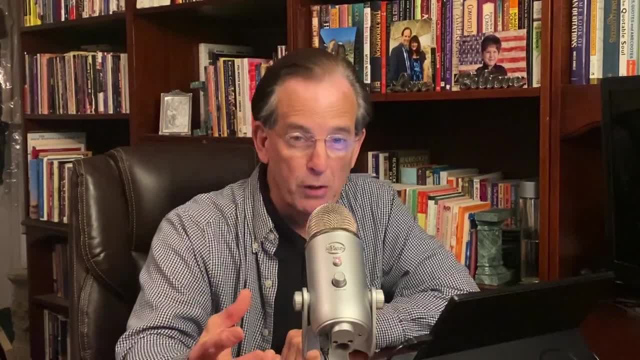 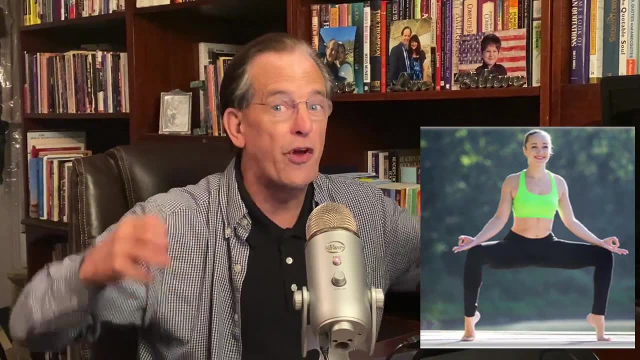 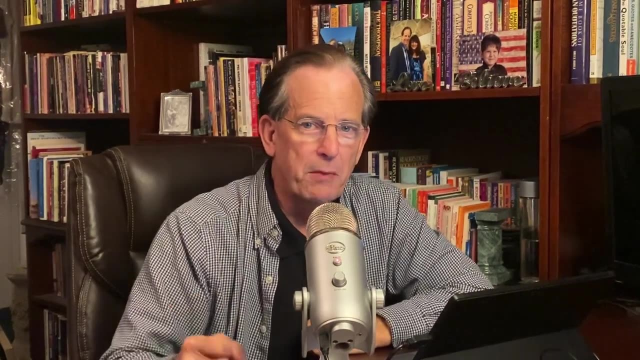 around her neck, which is a very fearsome looking deity, And when anyone in a yoga class assumes the goddess pose, they know they're tapping into goddess power to be fierce women, strong women, or at least many people who do it with the knowledge of what these 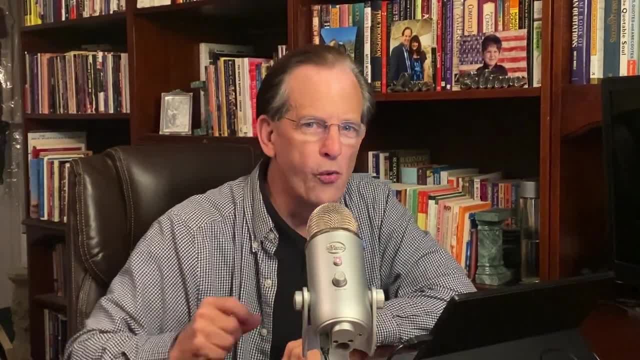 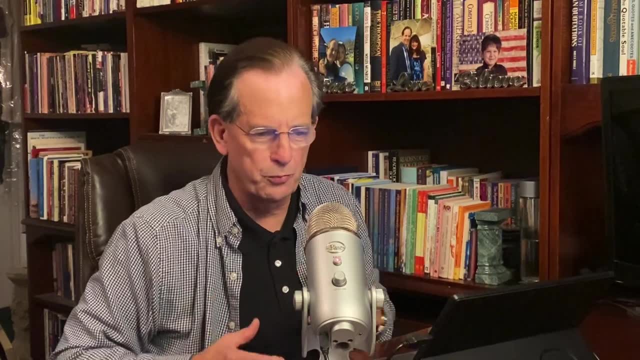 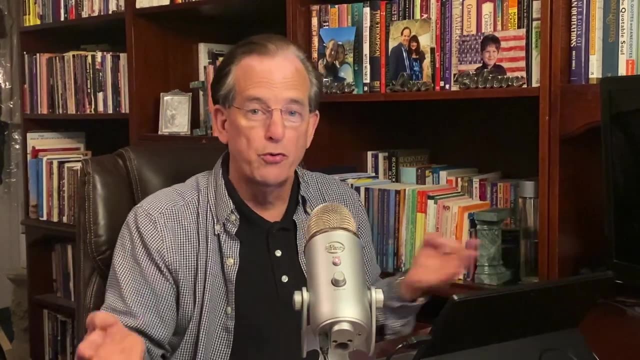 these postures mean will know that it's a connection to a spiritual power, And the way it looks is a person will spread both legs as far as they can to either side, squat down and rest their hands with a Gyan Mudra on their knees, with back erect Next. 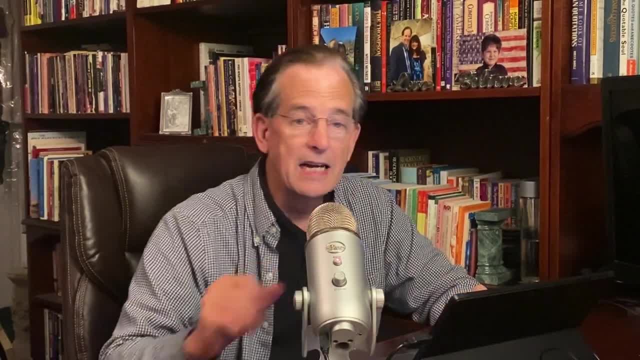 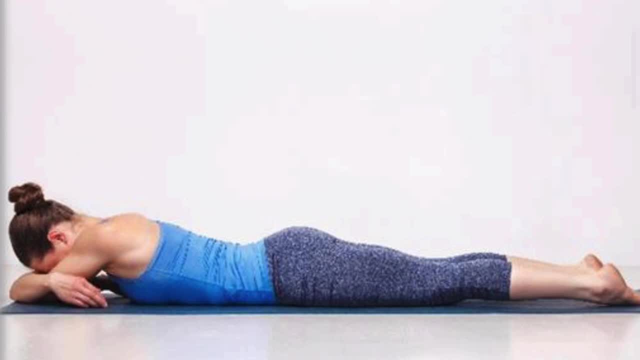 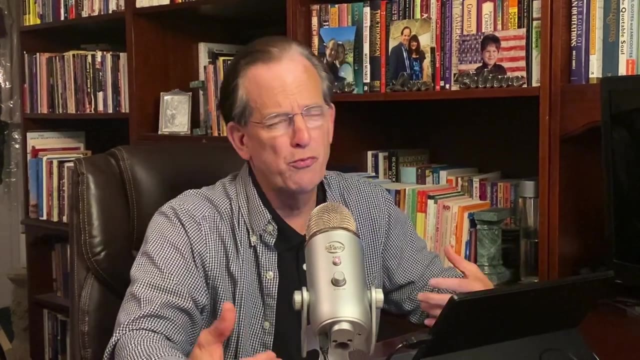 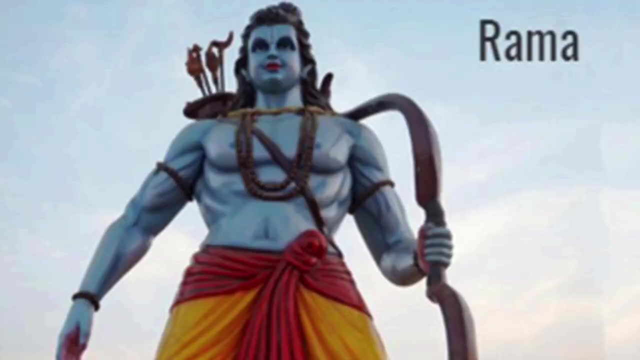 number eight is the crocodile pose. The crocodile pose is a very simple pose of just laying flat on your feet, And it's dedicated to a god who is respected as a god who represents morality and righteousness and good choices, a god named Rama, who was supposedly an incarnation of Vishnu or an avatar. 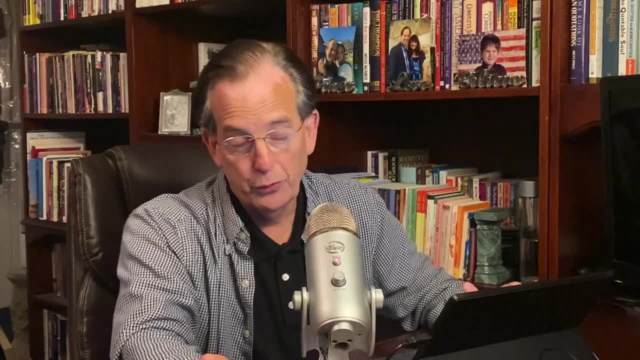 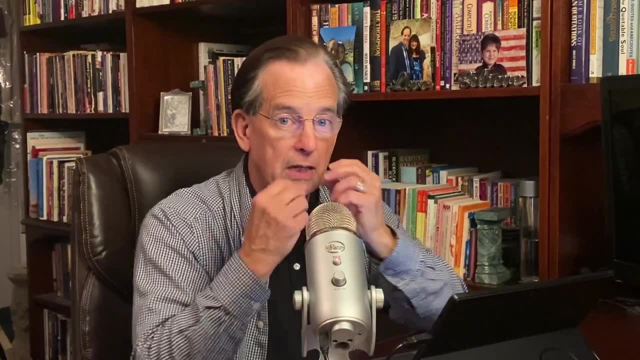 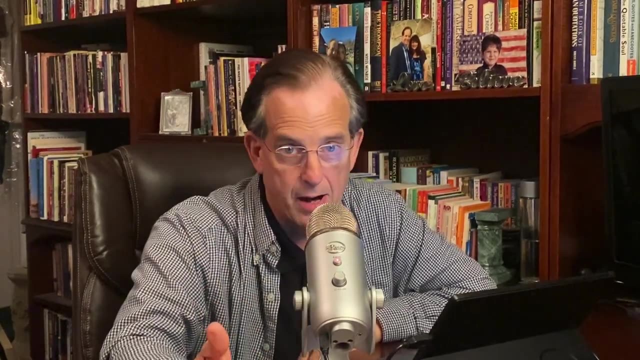 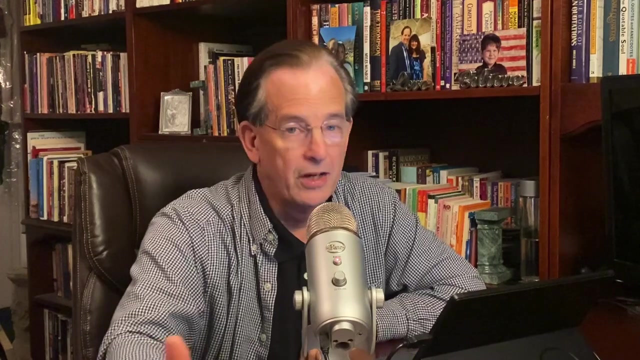 of Vishnu. I might include that the last word on Gandhi, on Gandhi's lips when he was assassinated, when someone shot him, the last words he said were Hey Rama. So apparently he was calling on the god Rama, which is an insufficient name. 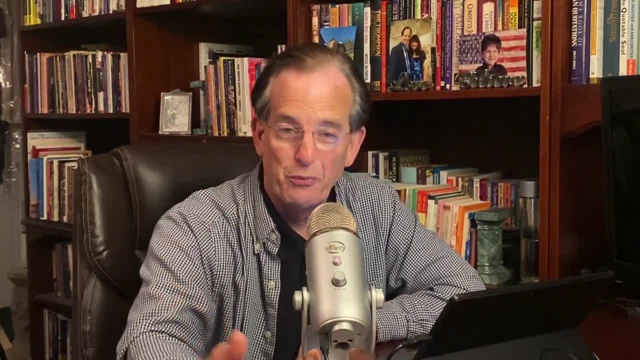 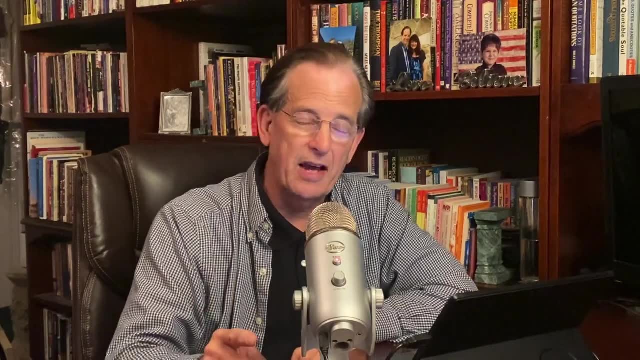 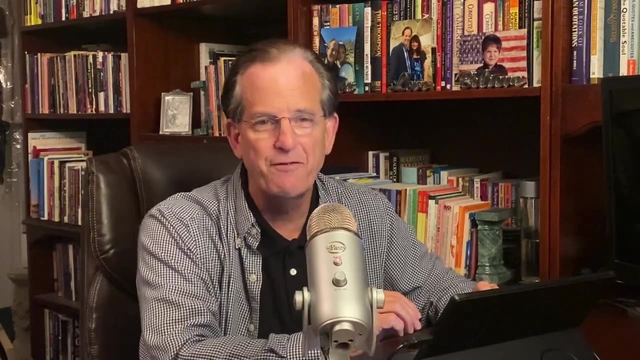 to step from this realm of time into the realm of eternity, because there's only one name that is above every name and the name by which every man must be saved is the name Yeshua or the name Jesus. That is the only name that connects you to the savior of all mankind. Number nine is the cat-cow. 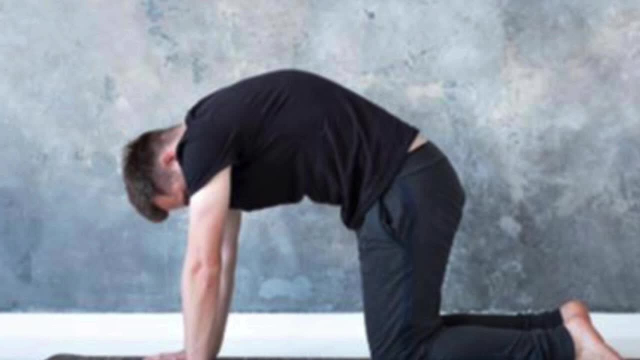 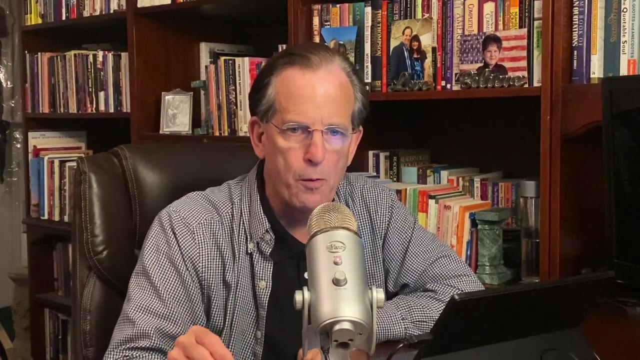 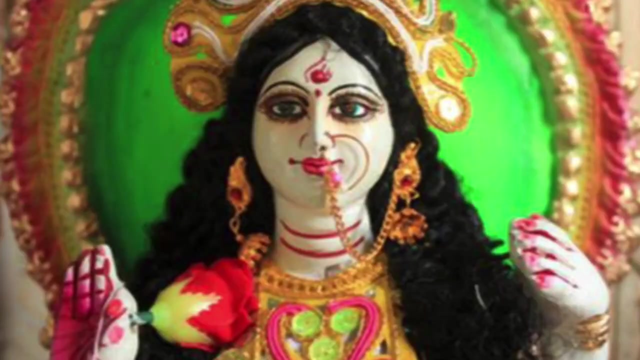 pose, And that's where a person first bends their back inward and then bends their back outward, And that's called the cat-cow pose on your knees and on your hands. That is dedicated to the goddess Saraswati, which is the goddess of learning and education, a female deity. 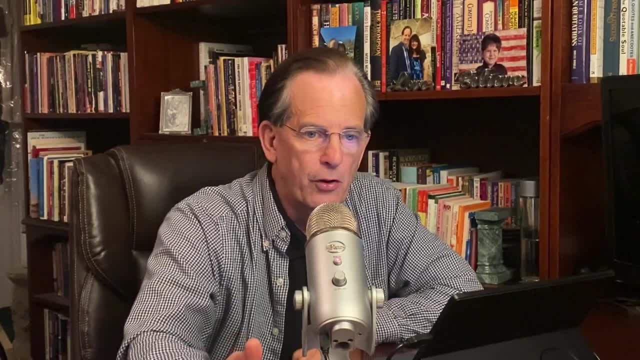 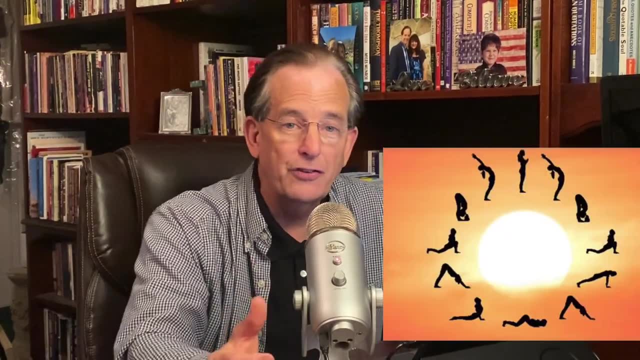 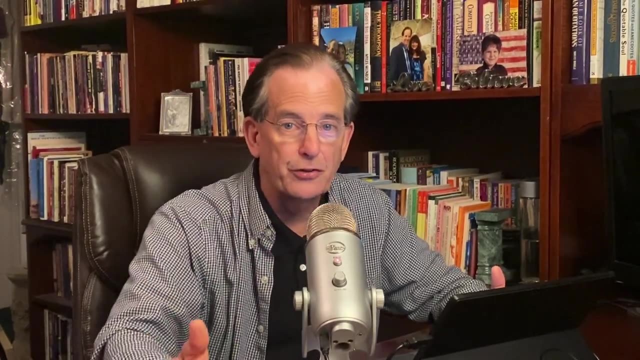 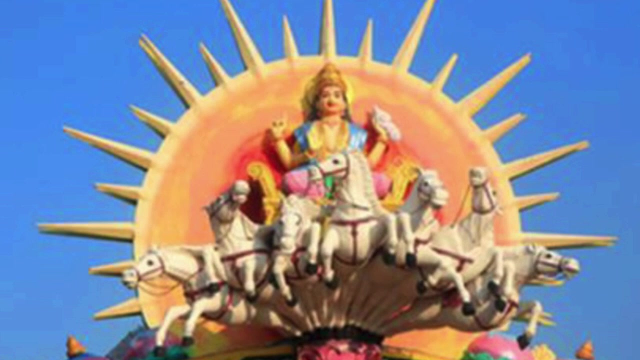 That is greatly respected among those who worship these deities. Next is the sun salutation, which usually begins a set of yoga postures, especially in the morning. It's a set of 12 different postures that are dedicated to Surya, who is the sun god. Now let me show you what the 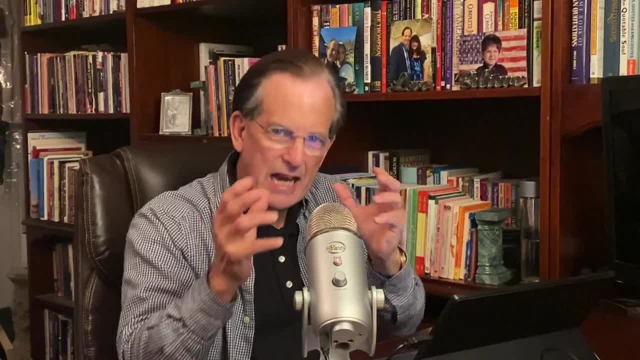 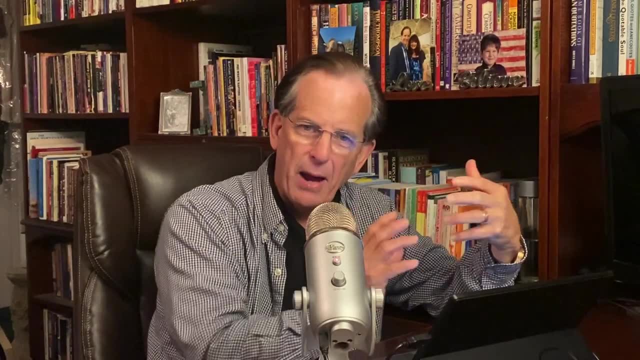 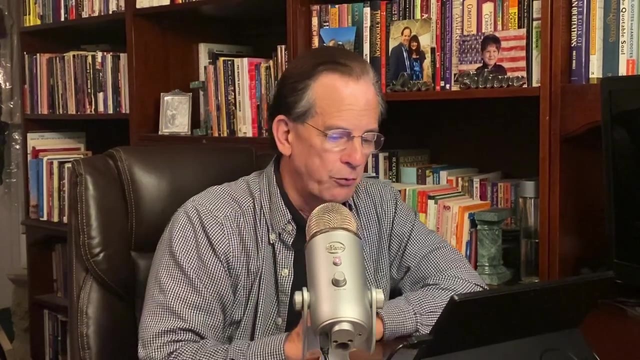 Bible has to say about connecting the creator with the creation, Worshiping an aspect of creation as an embodiment of the divine power behind it. In Romans, chapter one, verse 25,. in the complete Jewish Bible it reads this way: They have exchanged the truth of 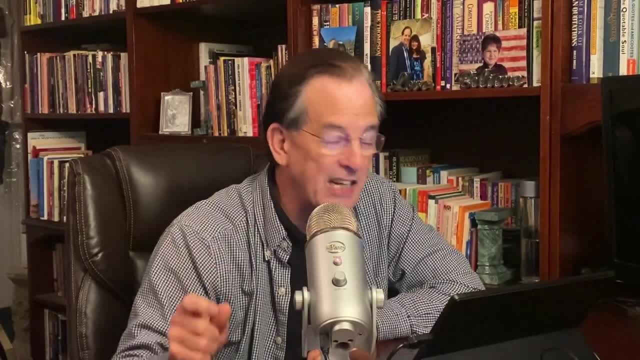 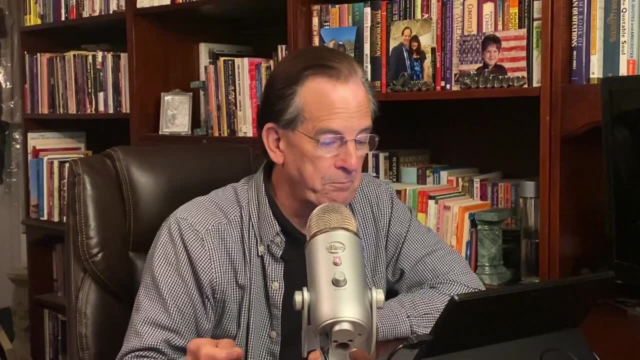 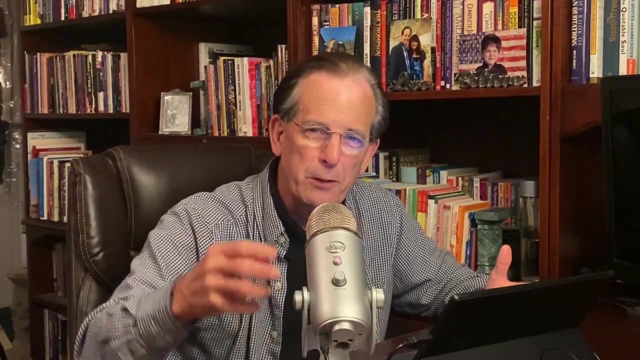 God for falsehood, by worshiping and serving created things rather than the creator. Praise be he forever, Amen. And so they exchanged the truth of God for a lie, For falsehood, by worshiping created things as an embodiment of the creator. Because see. 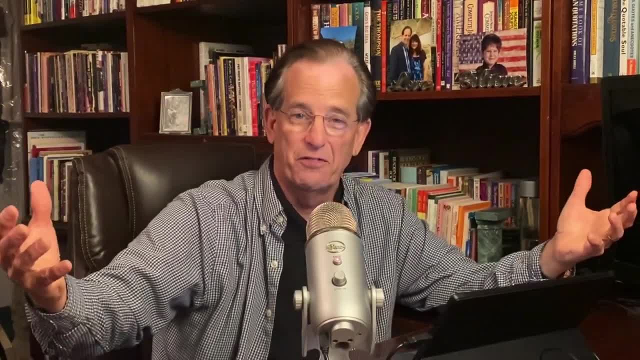 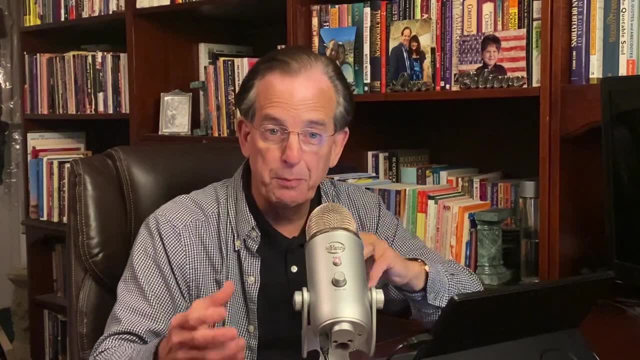 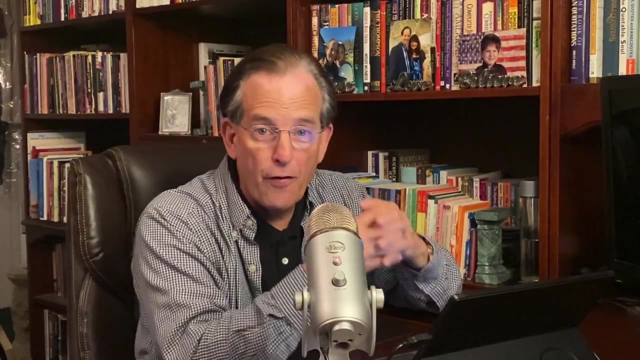 in Hinduism, the universe is a manifestation of the Godhead, So everything contains a divine essence, And because of that, many times, worship is connected to physical aspects of the universe. There's a goddess that is connected to the earth itself: Gaya. All right, let's go to the 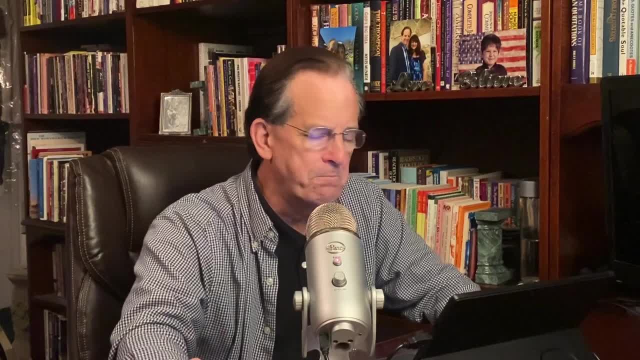 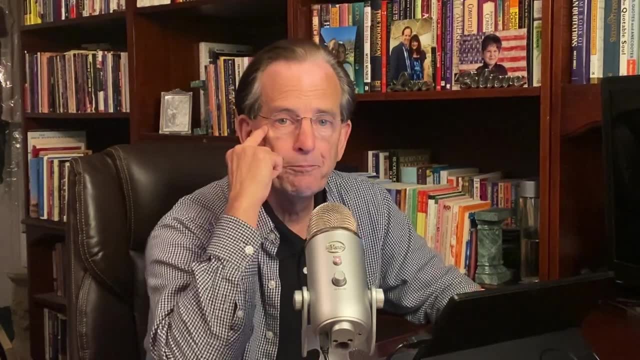 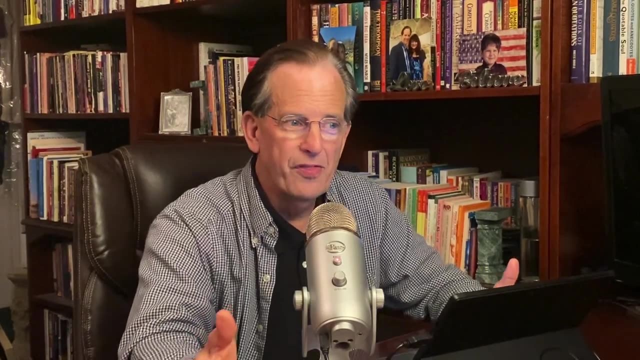 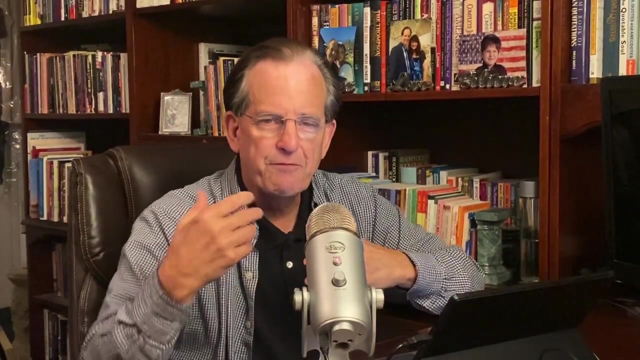 scripture. The scripture says that deal with the idea of these yoga poses being offerings to Hindu deities. See, I've been in India. In fact I've been in Hindu temples in India where they have a stream, a crowd of worshipers coming through the temple, laying flowers and fruits at the feet of these. 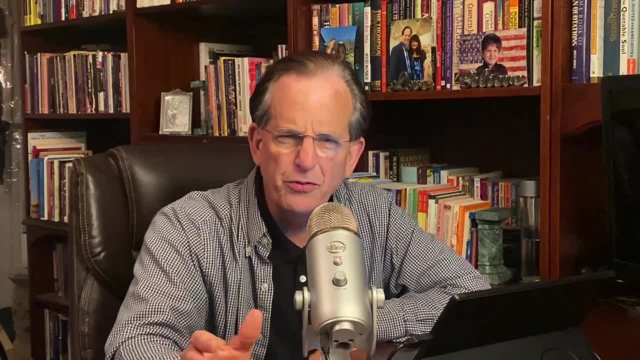 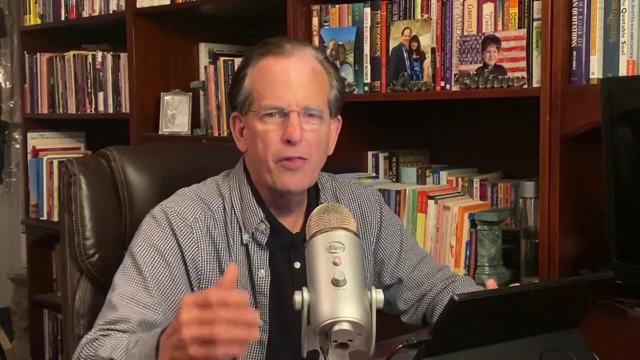 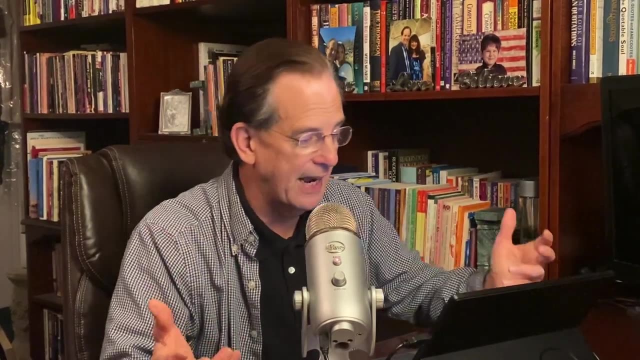 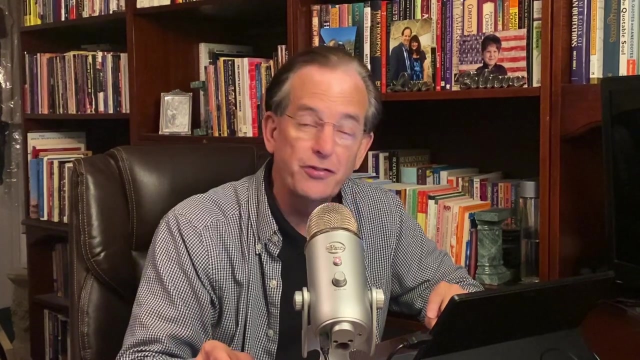 wooden and metal forms That are representative of gods and goddesses to them. And what did Paul say about that? Whether it be a yoga posture that is an offering to the deity, or flowers and fruits that are offerings to the deities, What does the apostle tell us? He said: what am I trying to say in 1 Corinthians 10,? 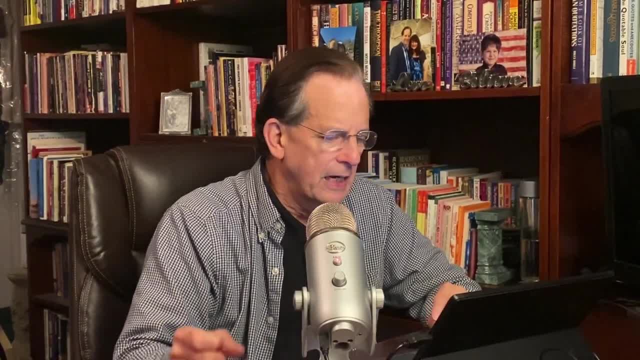 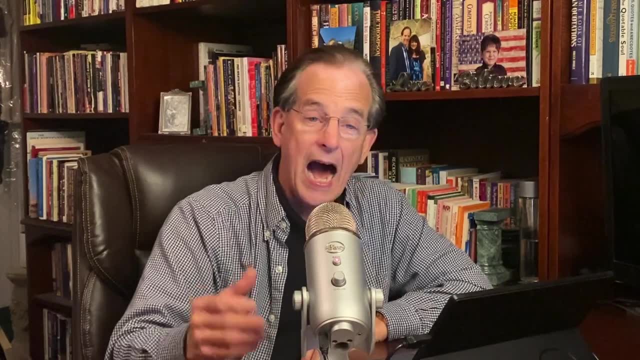 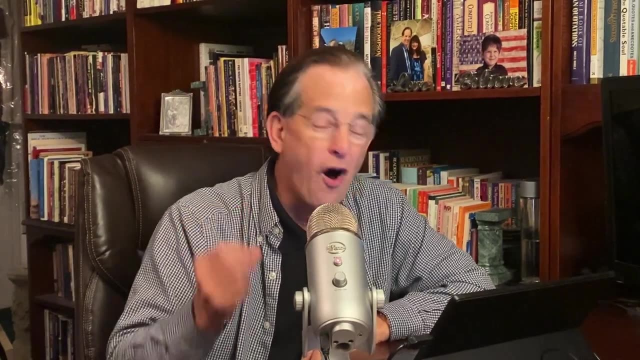 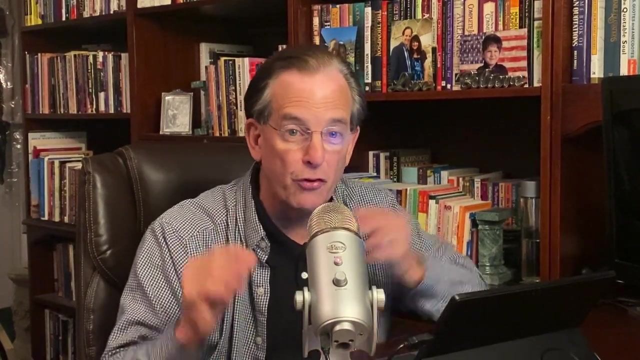 19 and 20 in the New Living Translation. He said: am I saying that food offered to idols has some significance or that idols are real gods? No, not at all. I'm saying that these sacrifices are offered to demons, not to God, And I don't want you to participate with demons. So now, 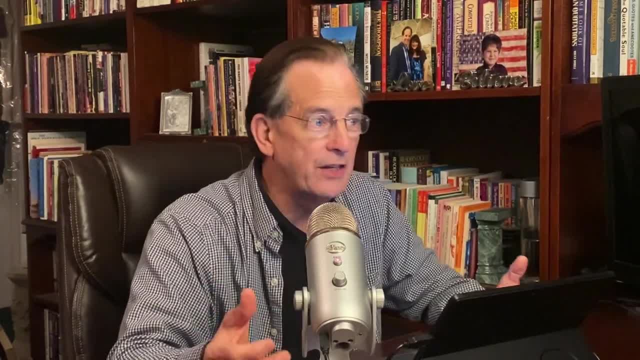 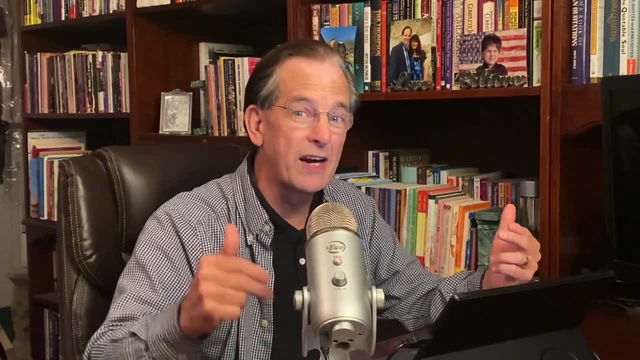 it's getting more serious. It's not just trying to connect with an imaginary deity that doesn't exist, but you are connecting with a demon, And I don't want you to participate with a demon. I don't want you to participate with a demon. I don't want you to participate with a demon. 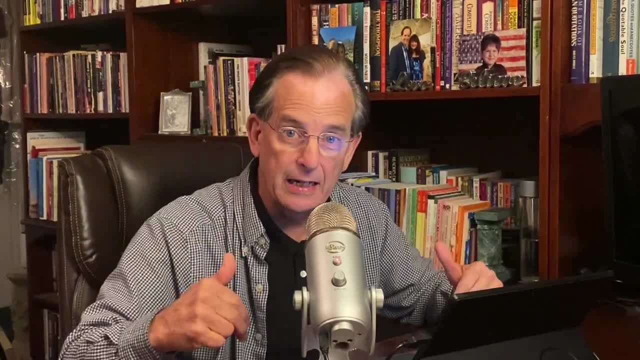 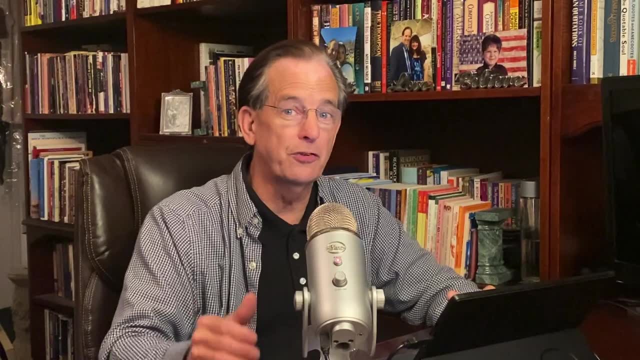 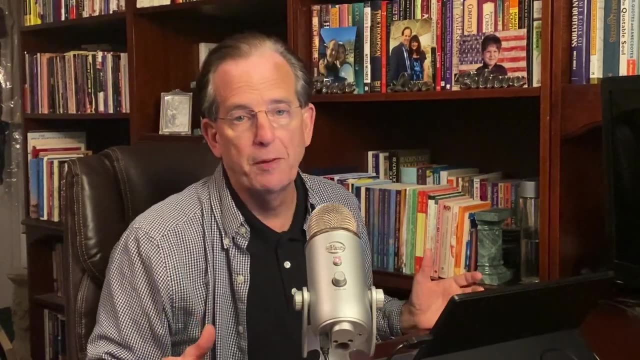 or demons that are impersonating those deities. No wonder people who do yoga, people who participate in yoga classes, may unknowingly have encounters with demonic forces. I've had people call me from around the world, desperate because they just started doing yoga, thinking that it was physical. 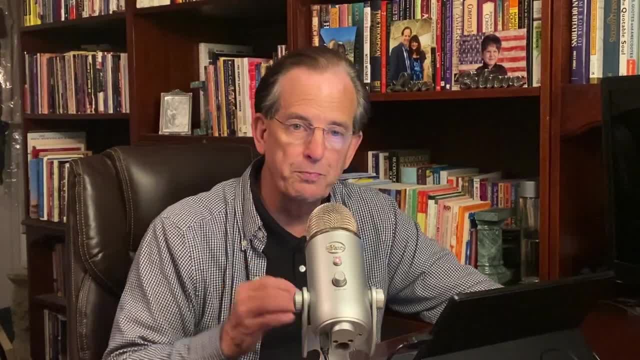 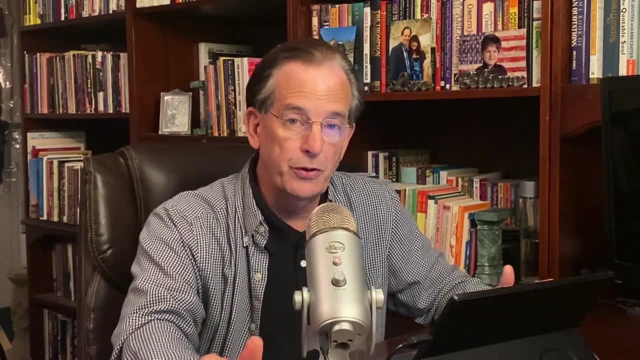 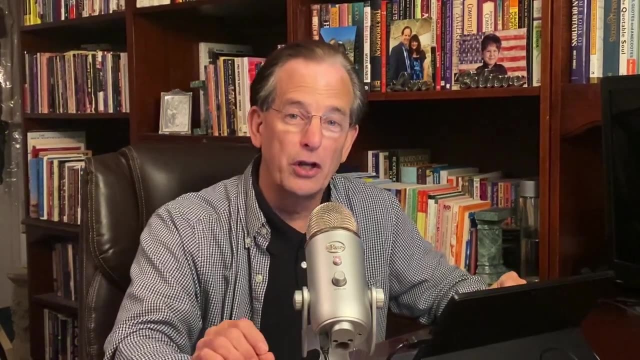 exercises, and they started having something called spontaneous kundalini awakenings, and I'm going to touch on that in just a minute. First, I want to share with you, though, before I get into what the kundalini is, that the deity that is referred to as the lord of yoga. the lord of yoga. 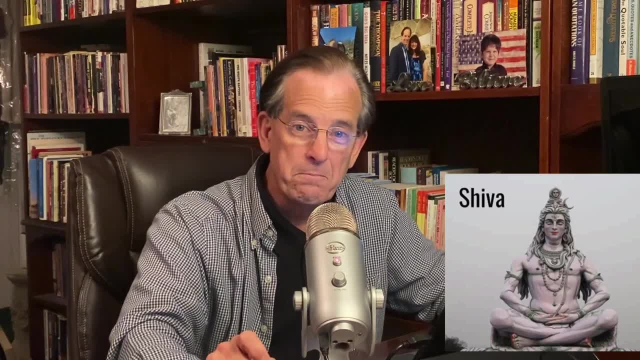 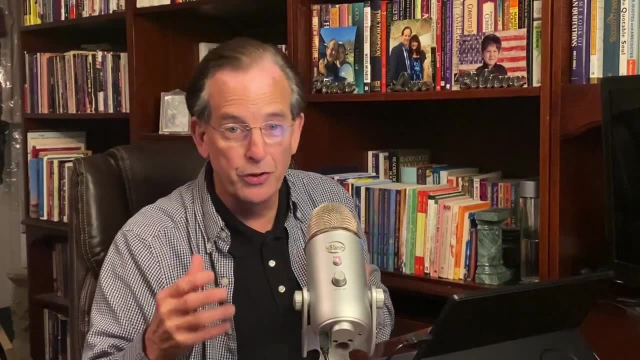 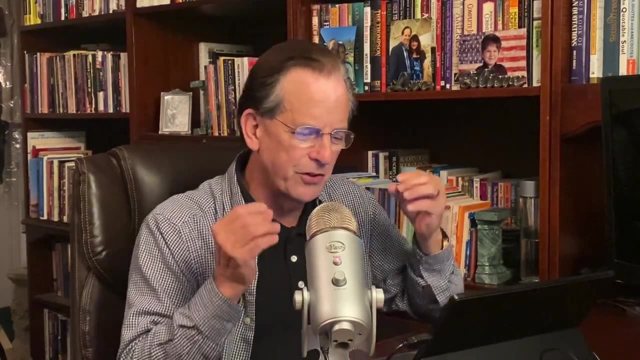 is the destroyer, god Shiva, and so there is a definite connection between Shiva and and and anyone who is a yoga advocate, whether it's recognized or not, whether you are consciously aware of it or not. there's a spiritual connection there, And see people when they do yoga. 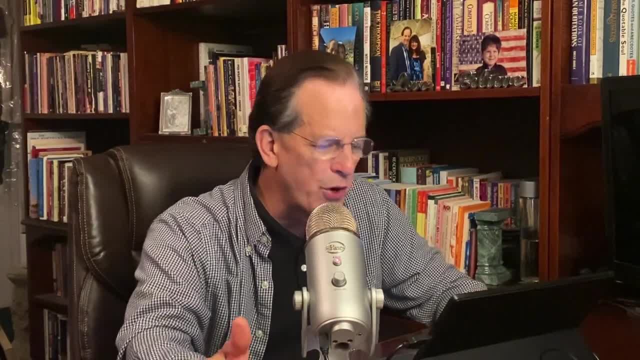 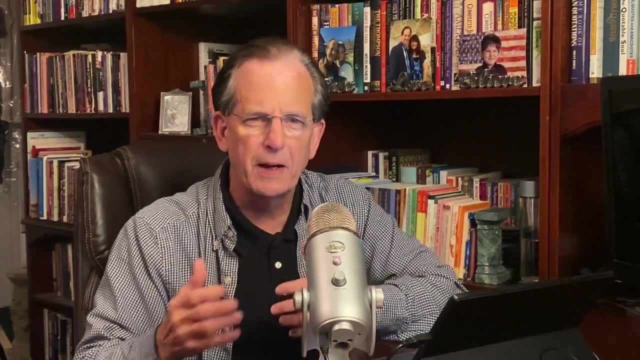 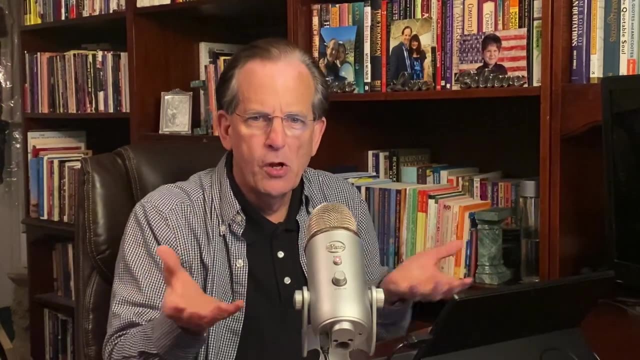 don't realize that the very word yoga means union. It comes from a Sanskrit word that means yoke and the implication is union, that your whole desire is to come into union with the over-soul, with brahman, with ultimate reality, with god-consciousness, or what has been also called. 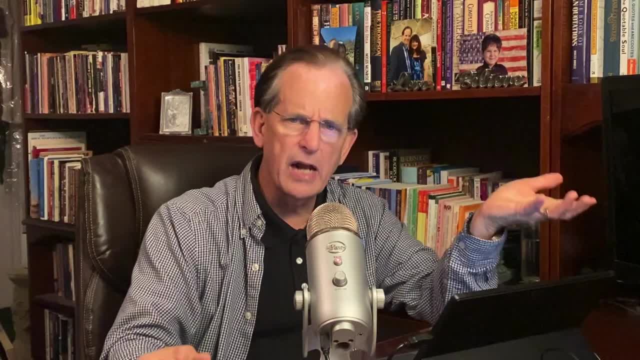 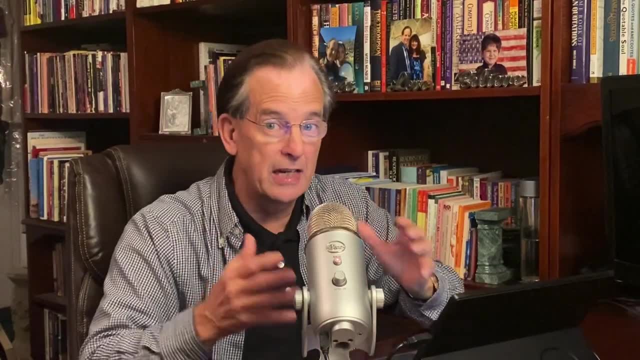 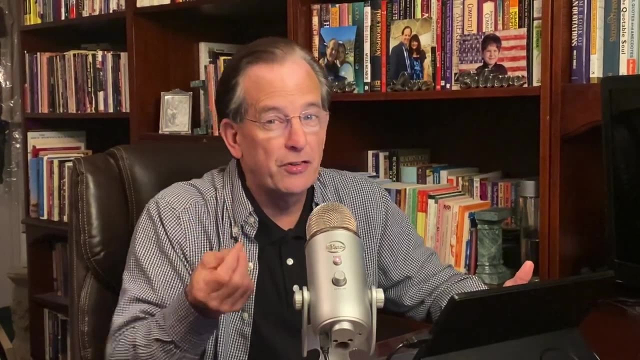 self-realization. Now, why would you call god-consciousness self-realization? Because within the ranks of those who believe this in Hinduism- and the vast majority of people who embrace Hinduism do- when you come to that ultimate experience of self-realization, you actually realize. 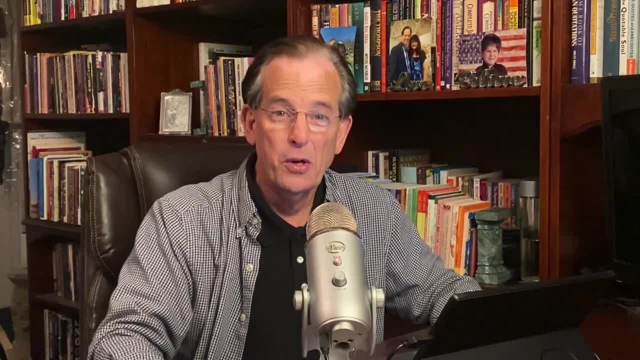 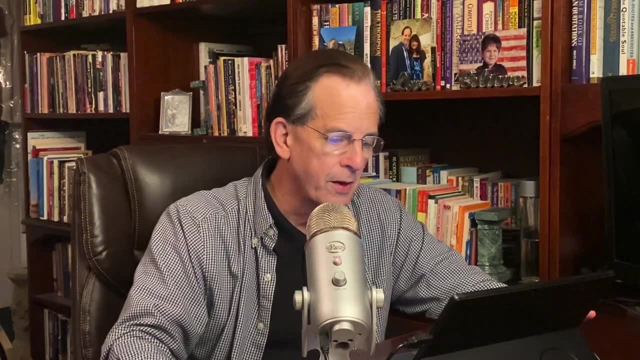 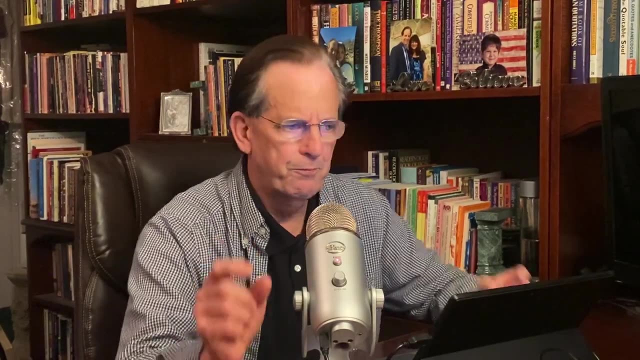 that you are a god, And so, when you come to that ultimate experience of self-realization, you are a god, which is the absolute antithesis of the truth. It's the absolute opposite of the truth. So what about this thing called the kundalini? See the main purpose for hatha yoga, which is 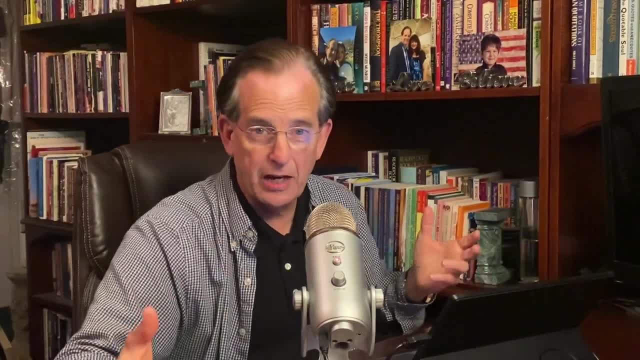 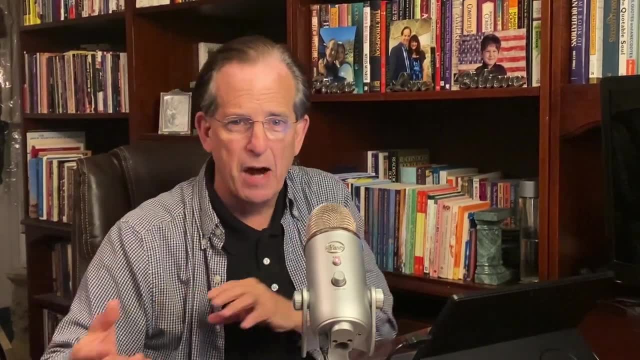 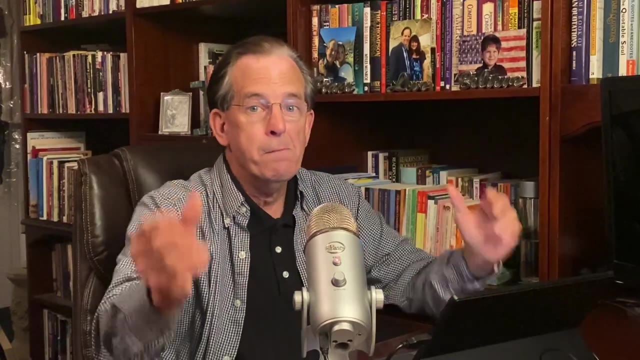 made up primarily of asanas, which are physical exercises, and pranayama, which are breathing exercises, where you don't get into the chanting of mantras. you don't get into the chanting of mantras, you don't get into the raja yoga, the mental kind of perceptions that help you escape. 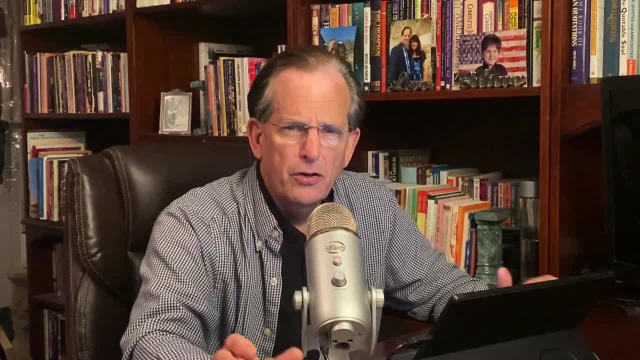 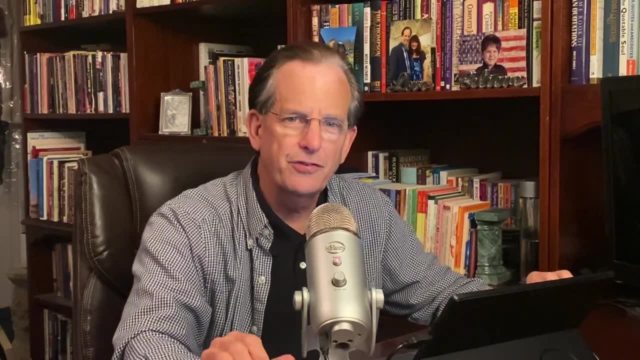 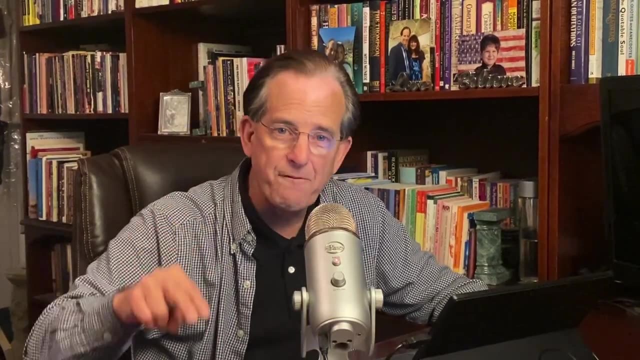 this world into a higher reality. You're just doing the basics, just doing the basics. now, Just pranayama, which is breathing exercises, and asanas, which are physical exercises. However they were created, They are the third and fourth limb of the eight limbs of yoga, according to. 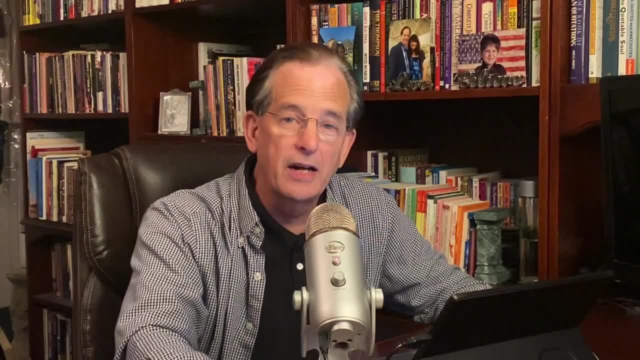 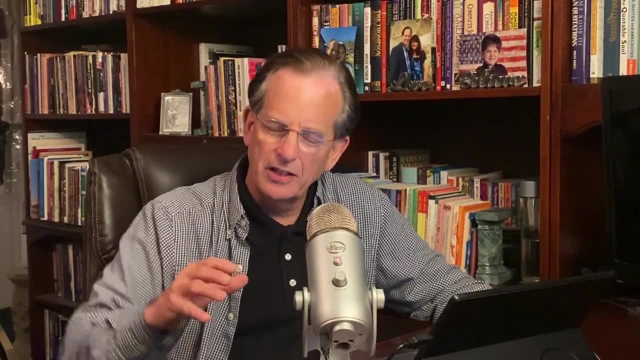 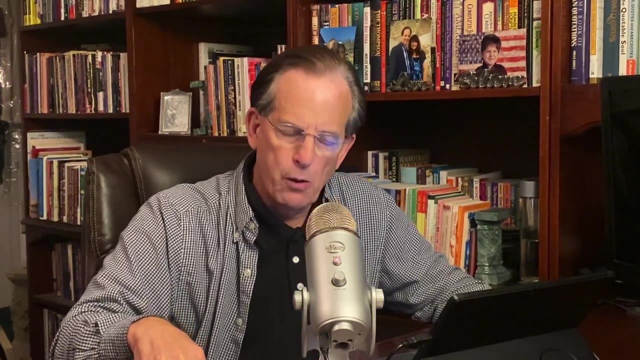 the kundalini, And it leads you to this state called god consciousness. Wow, this is really serious, See, the idea is that there is a dormant power at the base of the spine called the kundalini, And the word kundalini means serpent power, And when you do the yoga postures, it stirs. 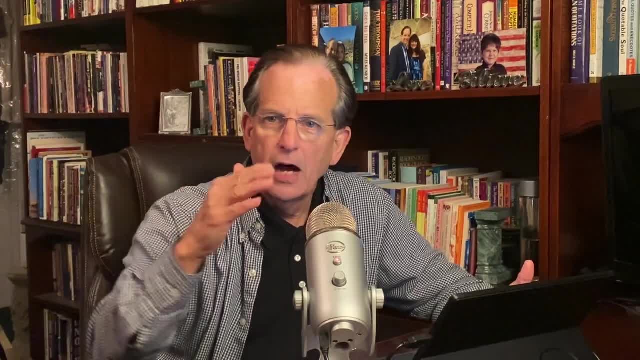 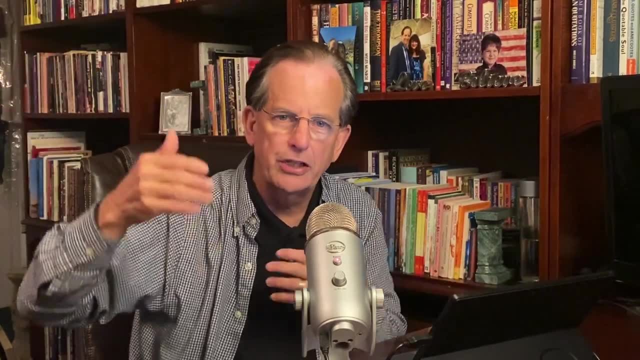 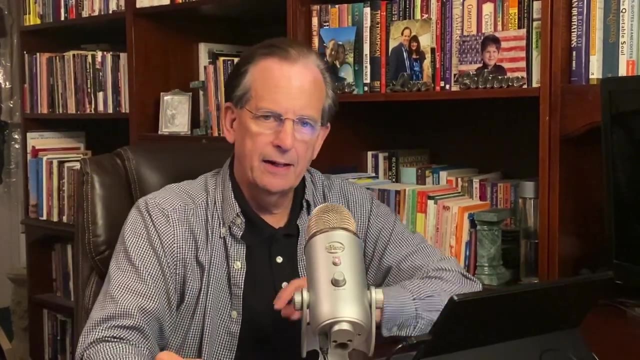 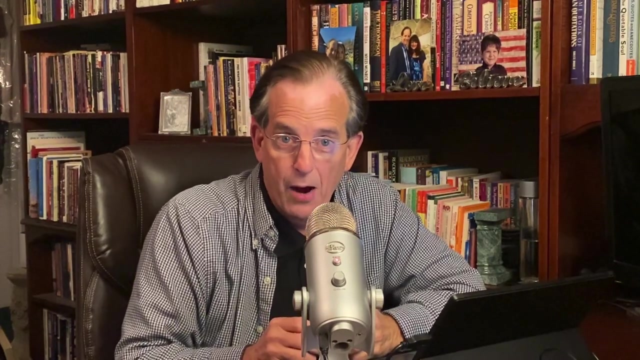 up that dormant power that then rises like a serpent up the spine, going through all the chakras- They're supposedly six energy centers leading up to the seventh energy center or chakra, which is called the crown chakra- And the teaching is that the power at the base of the spine is the shakti power. 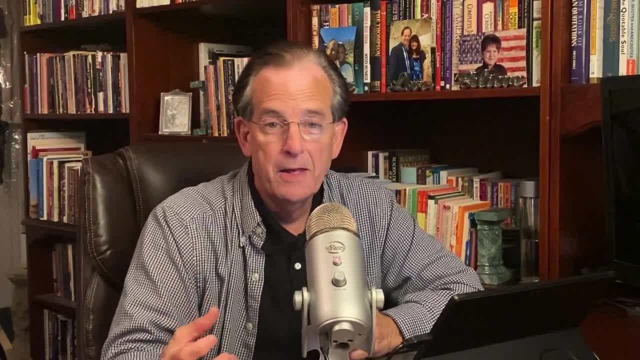 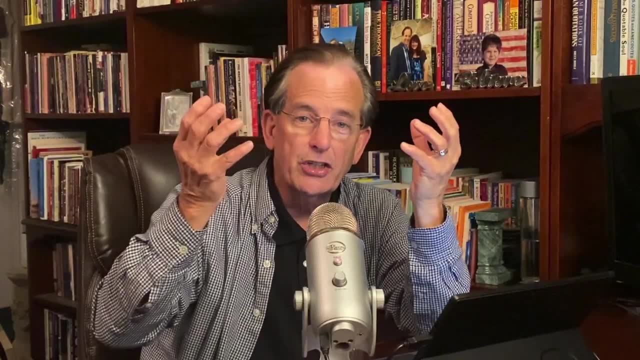 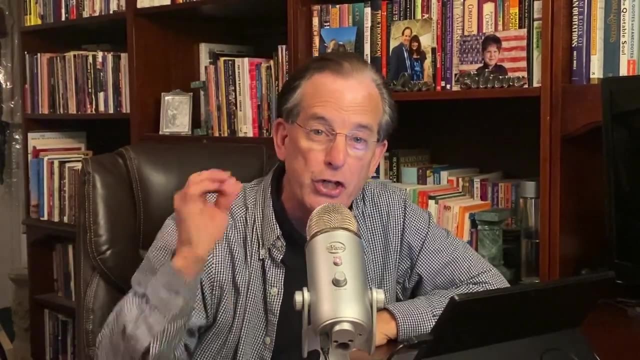 which is the female consort of Shiva. Shiva is the god of destruction And when the shakti power rises up through the spine, through the various chakras to the crown chakra, it merges with Shiva and you go out into oneness with God. You're yoked with that. God Know what happens, is you? 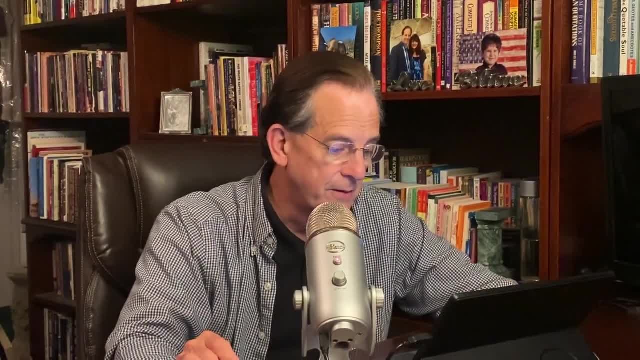 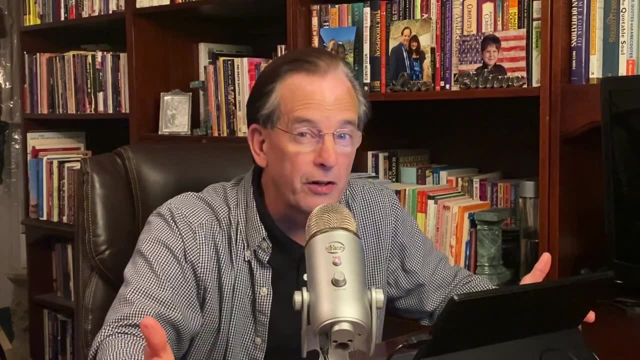 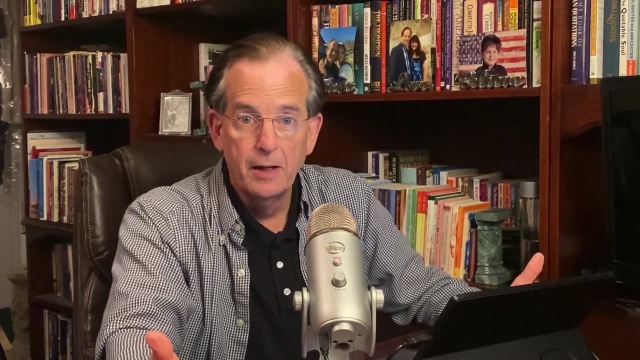 become demon possessed, which is a very terrible outcome of people that many times are sincerely trying to reach a peaceful place spiritually. They're trying to find fulfillment and wholeness spiritually, but actually they're opening themselves to a very dire situation And they're 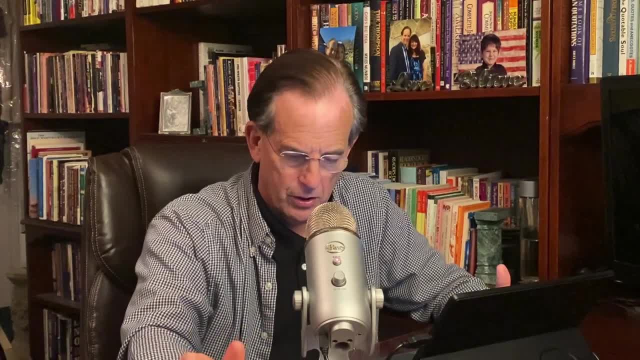 not there. They're there because they're going to fall victim And we pay attention to that And there's a question that I want you to look at. I'll give you five different responses to be on this matter, And particularly if they're going to be the ones who do this prayer. 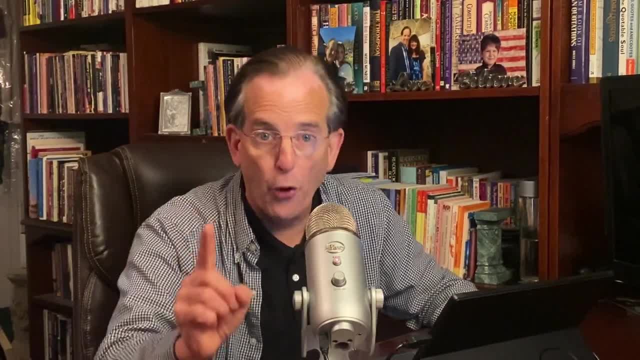 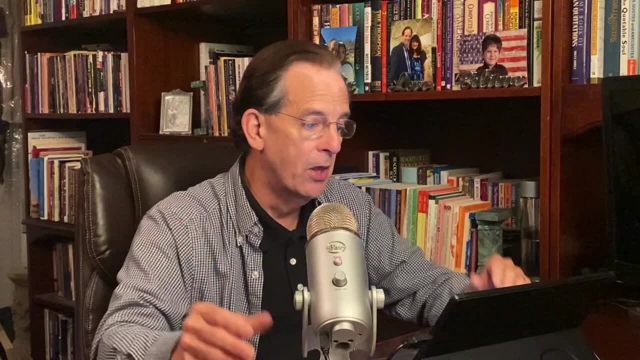 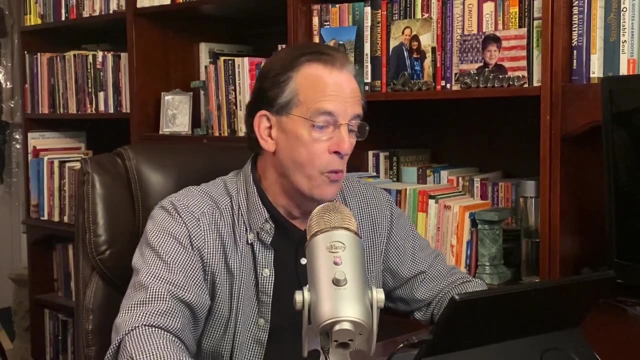 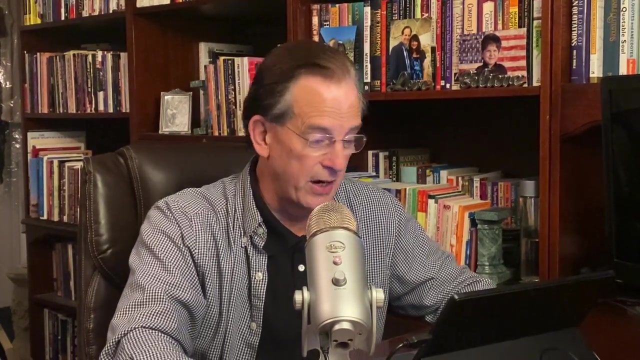 as well. I want you to get in contact with one of my religious disciples in the organization Bodhishan Chant Buldak. they're wielu-chudd tai. Do that attentively. I've taken it over several times with Belial. Or what part has a believer with an unbeliever? Or what agreement has the temple of? 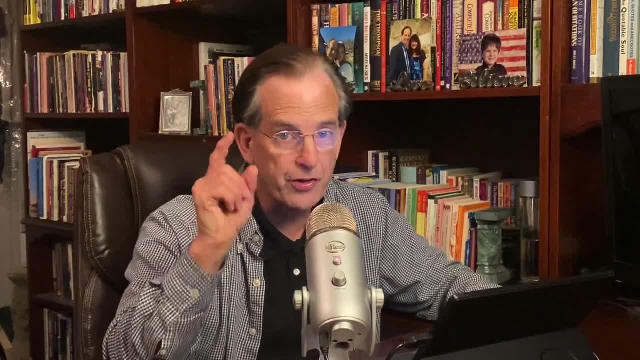 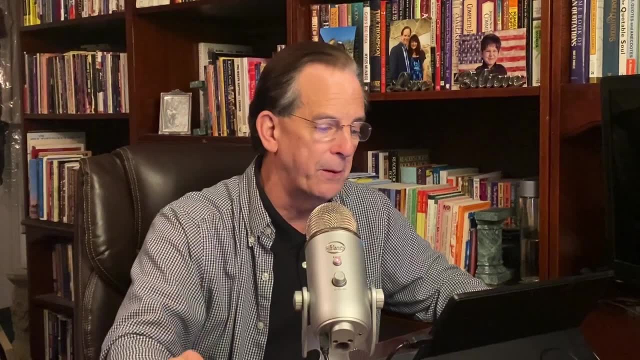 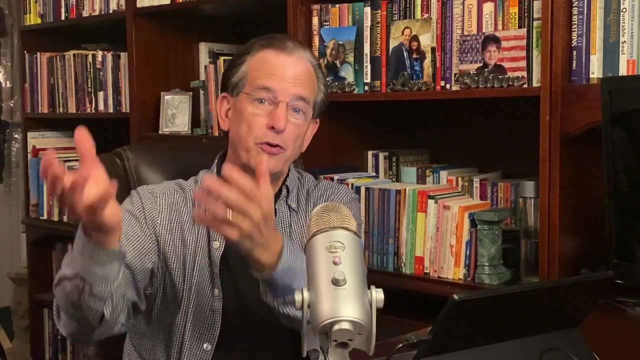 God with idols, For you are the temple of the living God And God has said: I will dwell in them and walk in them, I will be their God and they shall be my people. And I urge you to lay aside that yoke of yoga but assume this yoke that Jesus talks about in Matthew, chapter 11,. 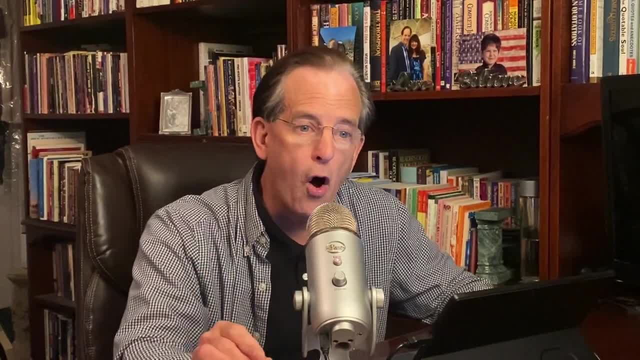 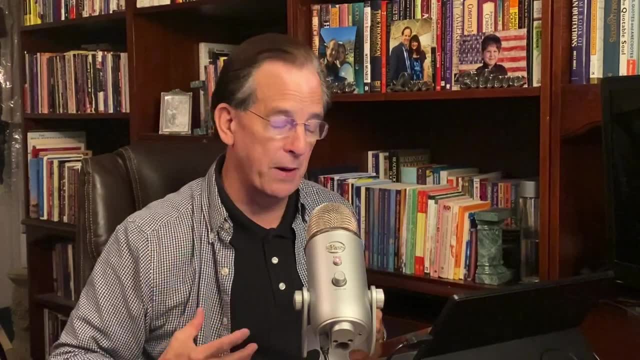 verse 28 through 30. He said: come to me, all you who labor and are heavy laden, and I will give you rest. Take my yoke upon you, which is the yoke of discipleship, the yoke of serving God the way. 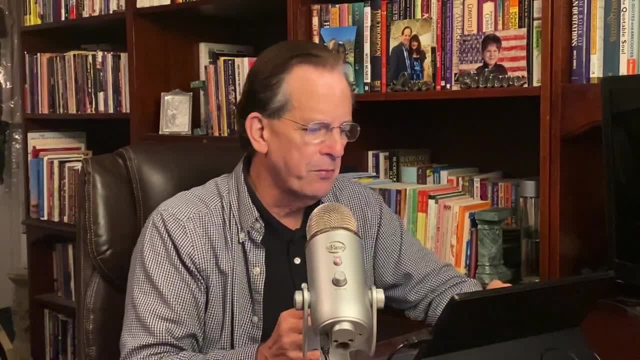 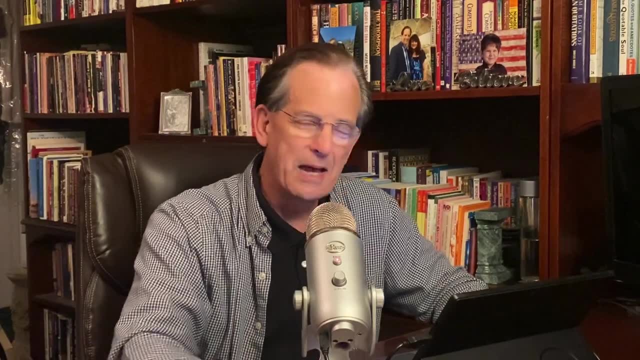 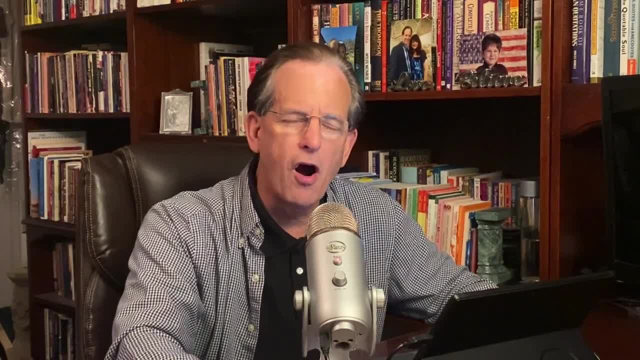 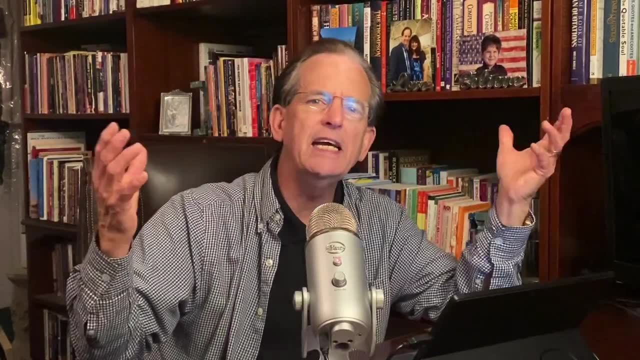 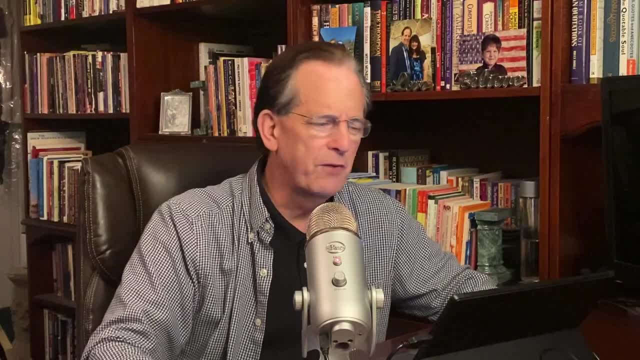 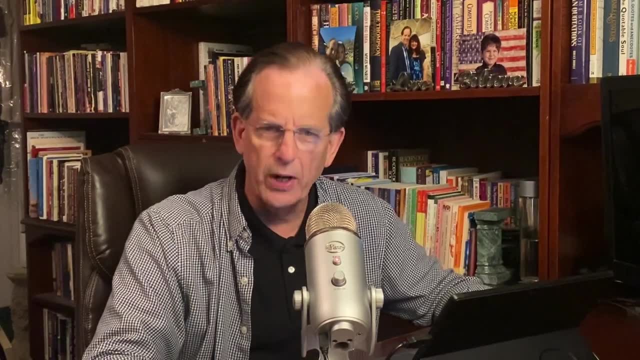 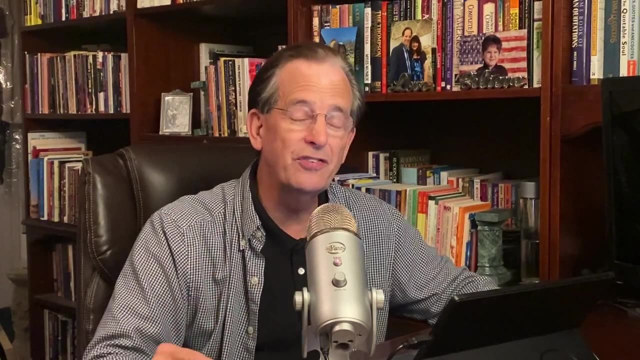 And it required intense discipline. We went from 3.30 in the morning till 5.30 in the afternoon every day, in some kind of yogic discipline, week after week, month after month, year after year, to achieve oneness with God. Jesus said: my yoke is easy, because all you're required to do is 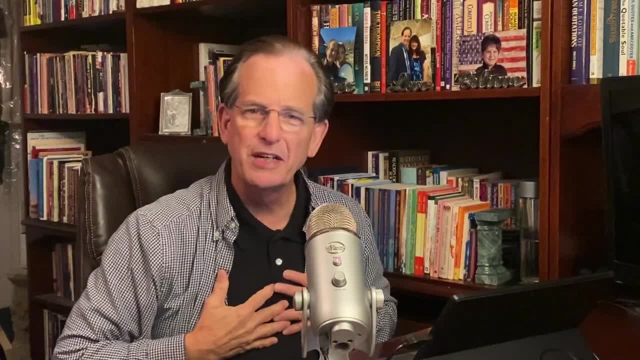 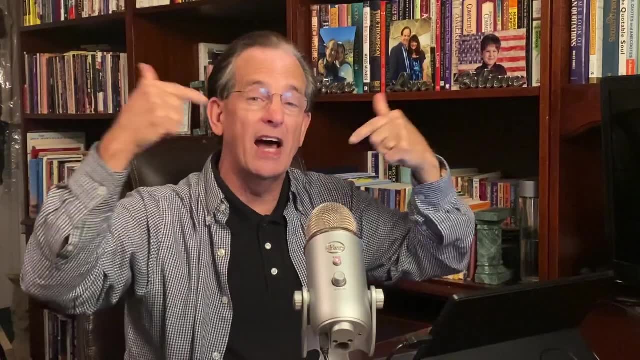 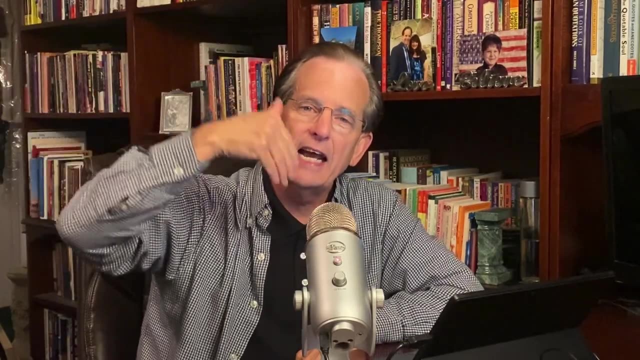 receive him as Lord of your life, Accept him into your heart- Ephesians 3.17,. Christ will dwell in your heart by faith, and you are born again when the Spirit of God enters into you. It's not a latent serpent power at the base of the spine, It's the Spirit of the living God entering into 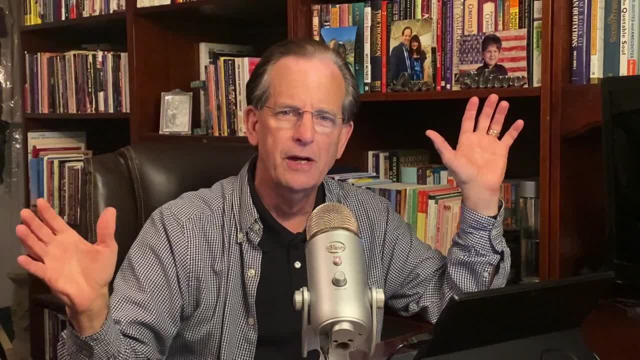 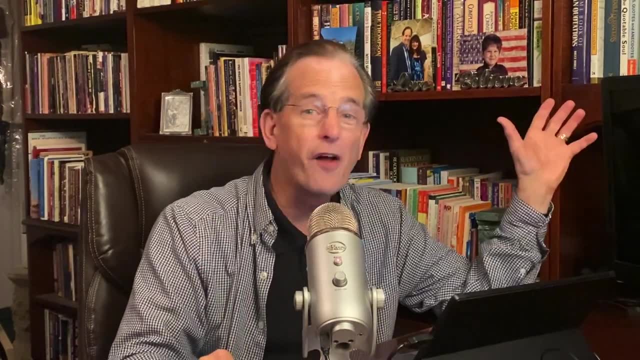 you from without. It's a completely different approach And you're born again and you receive the gift of eternal life. That yoke is easy. Discard the yoga yoke and take the yoke of serving the Lord Jesus Christ the rest of your life.